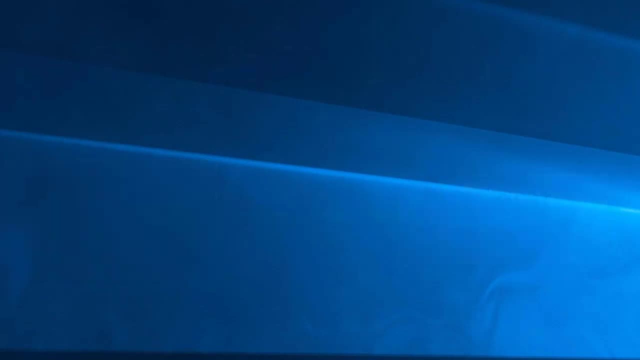 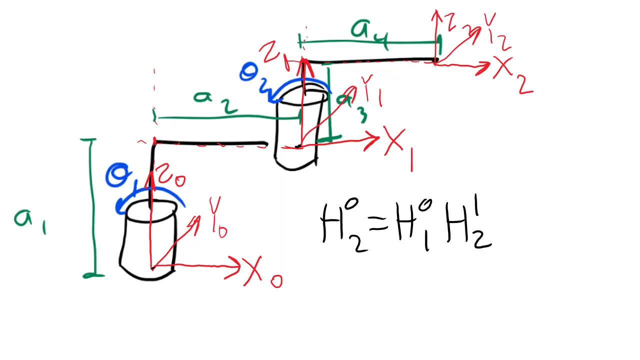 Inverse kinematics, as it turns out, is a somewhat more difficult problem than forward kinematics. Let me start by giving you a brief example of why inverse kinematics is difficult. Here I'm showing the kinematic diagram for the manipulator we've built. We know that we can. 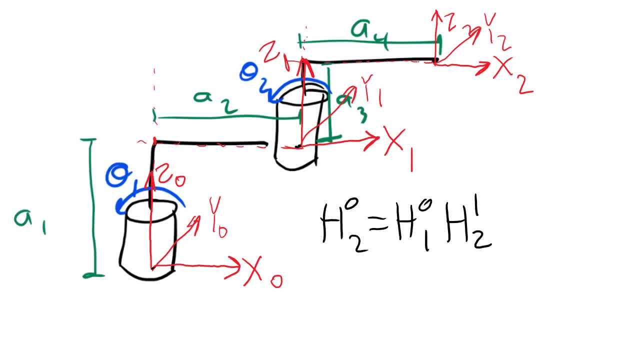 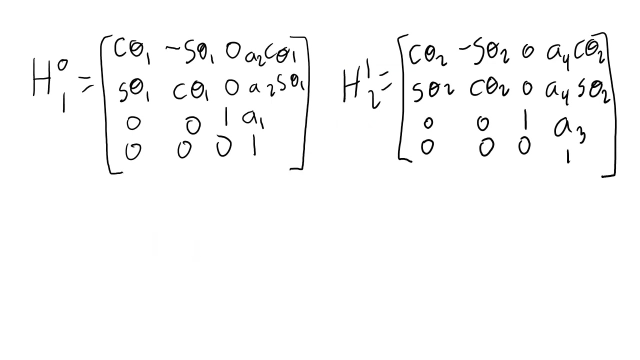 find the complete homogeneous transformation matrix from the base frame to the end effector frame by multiplying together the two, two individual homogeneous transformation matrices. In previous videos we've already found H01 and H12.. Let me remind you what those are. Now to get H02, I could do that by multiplying. 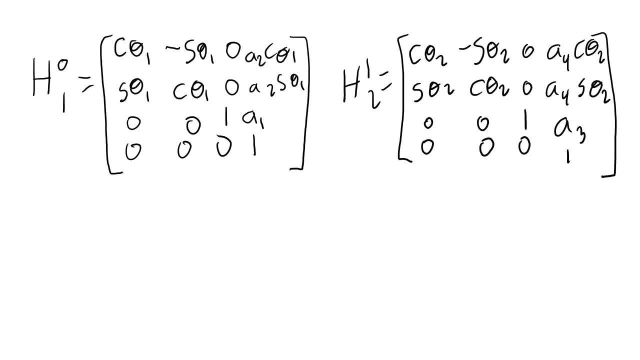 these two matrices together. In the past, we've stopped at this point and put these matrices into our code, But for this example, where I'm showing you why inverse kinematics is difficult, I'm going to multiply them by hand and show you the result. Here's the result of this multiplication: 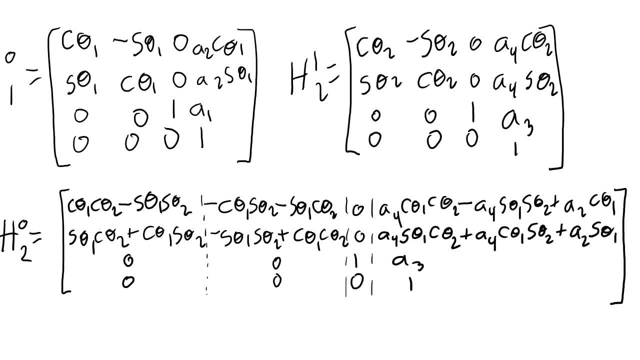 I drew dashed vertical lines to differentiate one column from the next. Remember that the homogeneous transformation matrix contains two points Parts. It contains the rotation matrix in the upper left-hand corner and it contains the displacement vector in the upper right-hand corner. In other words, the displacement vector is right. 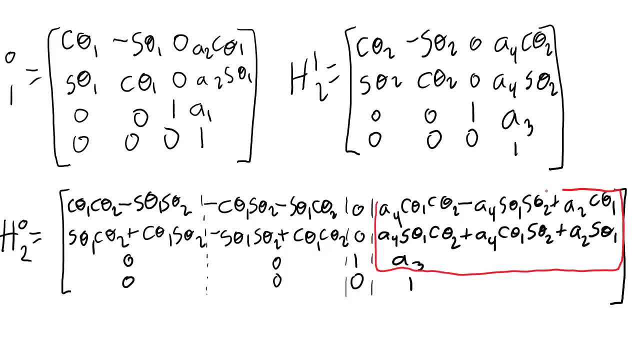 here. This first long crazy element is the x position of the end effector in the base frame. The second is the y position of the end effector in the base. The third is the z position of the end effector in the base frame. 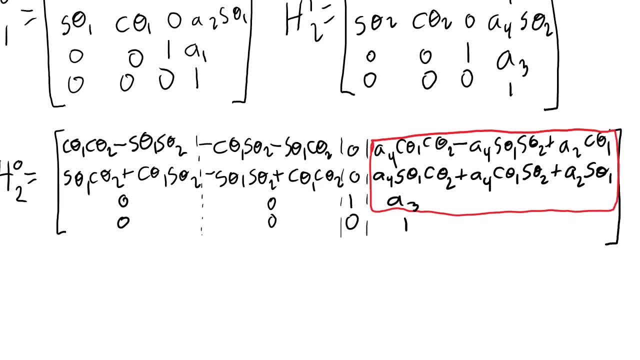 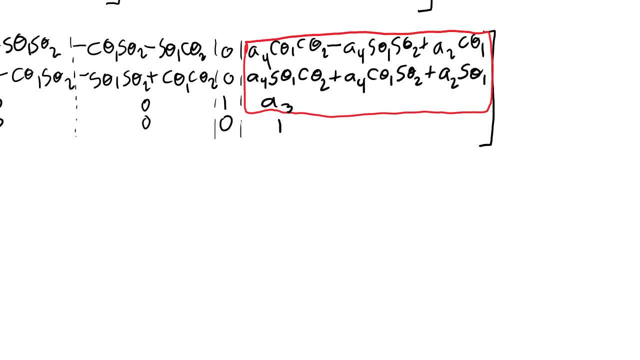 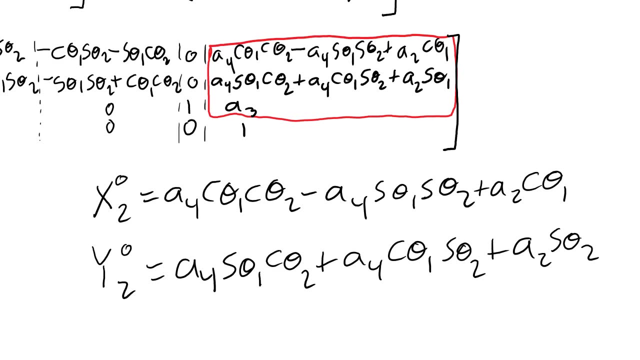 So let's suppose that I know the xy position where I would like the end effector to be. I could write out two equations like this: I simply take the first equation and set it equal to the x position where I want my end effector to be. 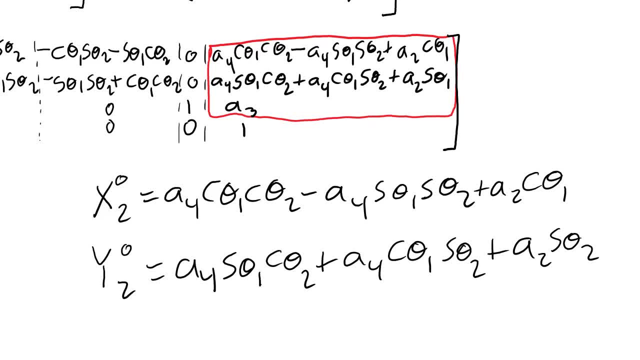 and I take the second expression and set it equal to the y position where I want my end effector to be. Now I could plug in two numbers for x and y and solve this system of equations for theta 1 and theta 2.. Do you see why this is a difficult problem to solve? 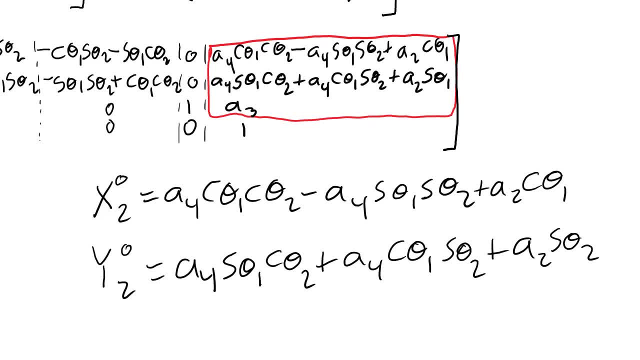 What we have here is not a linear system of equations, but a nonlinear system of equations, because of the presence of all of these sines and cosines in these two equations. The only way we could solve this problem would be to do some kind of numerical solution. 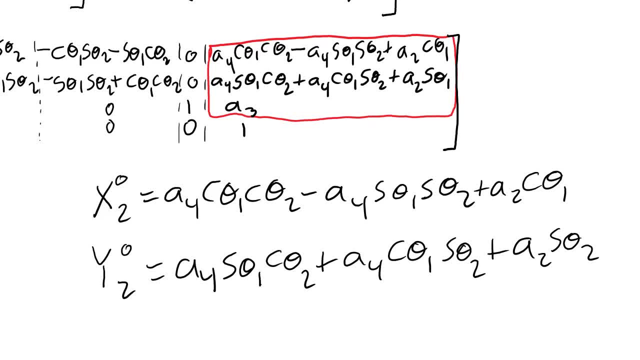 We can't solve it analytically. Actually, this is one valid way to do inverse kinematics: to write out these equations and then use a numerical method to solve this nonlinear system. But there is another method we can use to actually get an analytical solution, and that's 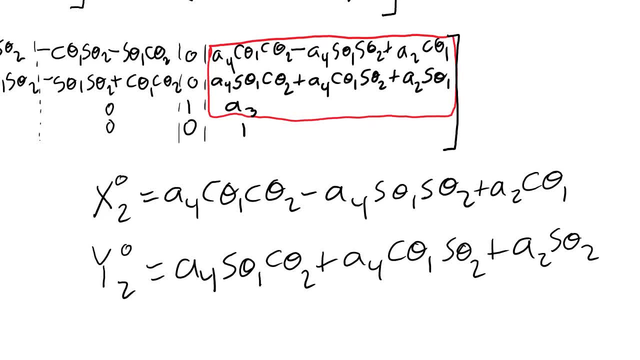 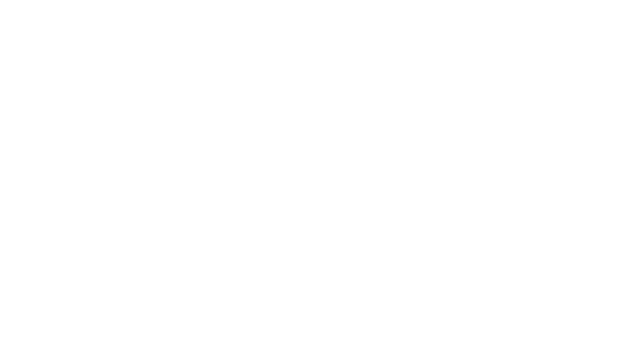 what we are going to be looking at today. This other method is known as the graphical method. I'm going to give you an easier example for the graphical method, before we go back and use the graphical method on the manipulator that we've built. 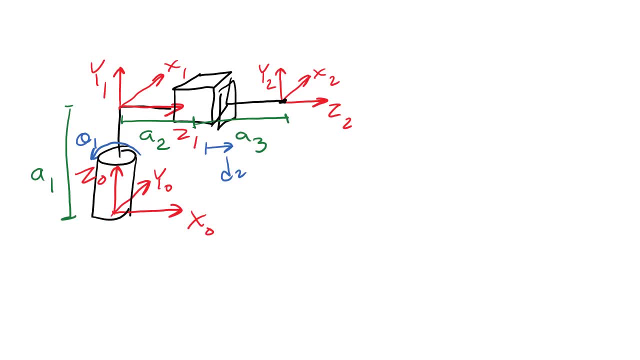 Let's suppose that we want to do inverse kinematics On this two degree of freedom manipulator. In other words, we want to be able to specify an x, y, z location for the end effector and we want to solve for theta 1 and d2.. 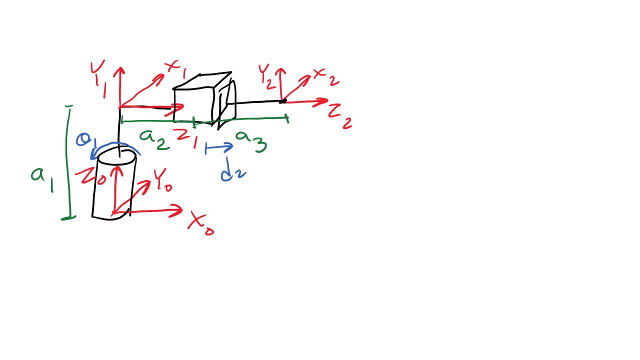 We're going to start the graphical method by drawing this kinematic diagram from two different views: Either the top view, That is, drawing the Kinematic diagram in the x y plane, Or the side view. In the side view, we just want to be able to look at the manipulator in a plane that. 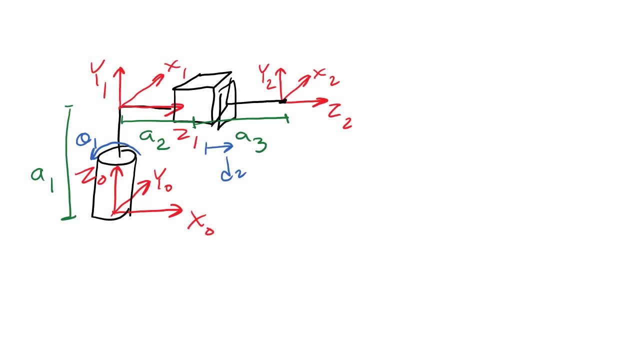 includes the z axis. So for this example, we're going to start by drawing the manipulator in the top view. That is, looking at the manipulator as if we're looking down from the top and seeing the x- y plane. So when we 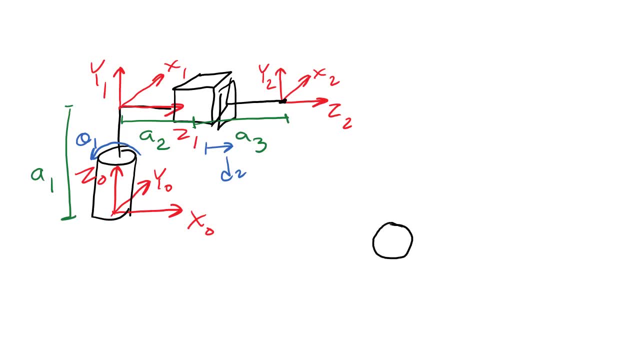 Look down from the top, we'll see the top of this first joint looking like a circle, like that. We'll see the x zero axis pointing off to the right And we'll see the y zero axis going up to the top. Now it's important when we're doing this graphical method that we draw the joint variables, not 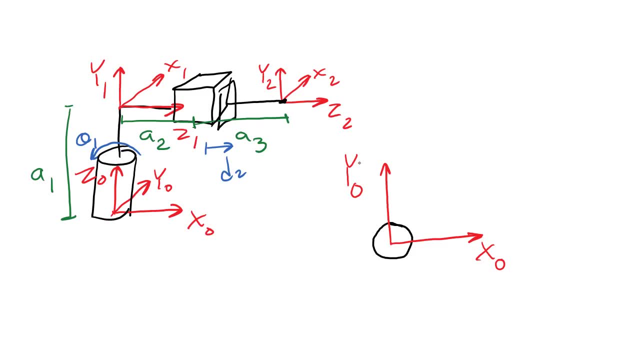 in their zero position And in fact, we also don't want to draw them In A position like 90 degrees or 180 degrees. We'd prefer to draw them in a position like 45 degrees. That will make it much easier for us to solve this problem. 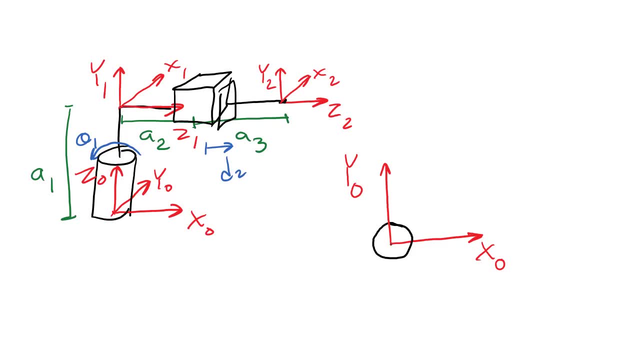 So if theta one was at 45 degrees, we would see its link, a two pointing Like this. Then we would see the second joint from the top looking like a Square And the last link in the end effector right here. Now I'm going to draw in. 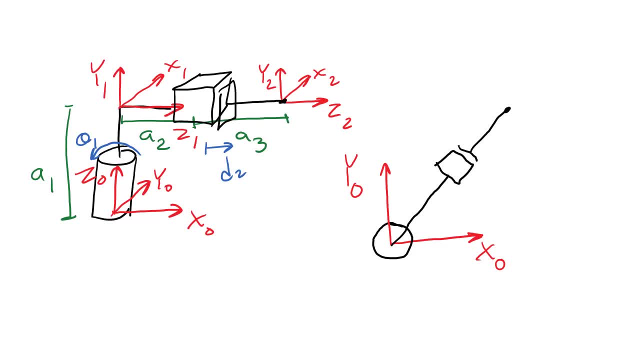 The link lengths and the joint variables into this top down view. In this top down view, this angle here is theta one And d two is over here. This angle here is theta one And d two is over here. This angle here is theta one. 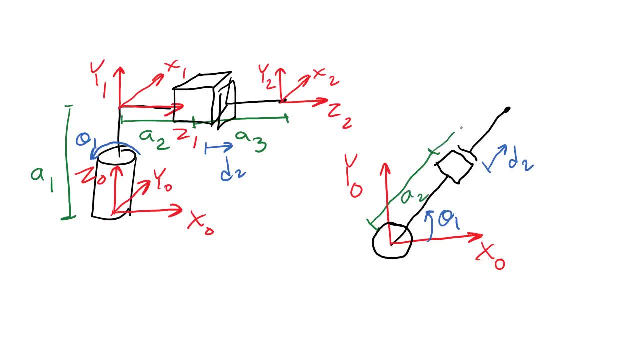 This distance is the link length, a two, And this link here is a three. Now the graphical approach to inverse kinematics relies upon us finding triangles that we can use to write relationships between the joint variables and the xy position of the end effector. 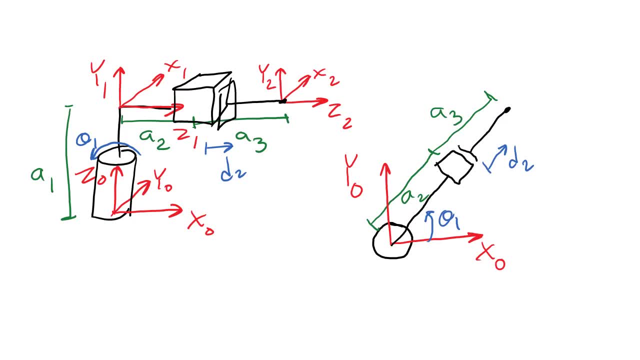 It takes a little bit of trigonometry experience And just some experience solving these problems to help you see which triangles are going to be useful. One of the triangles that is basically always useful is this triangle that I'm drawing in purple right here. 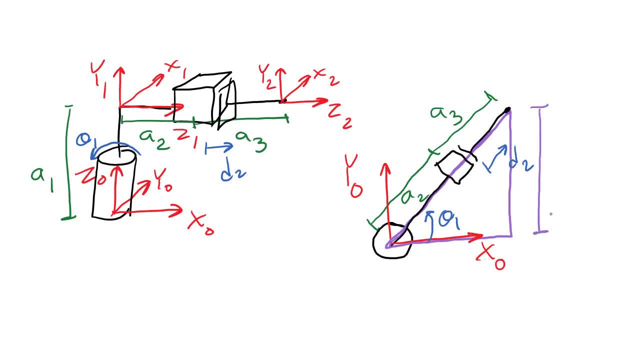 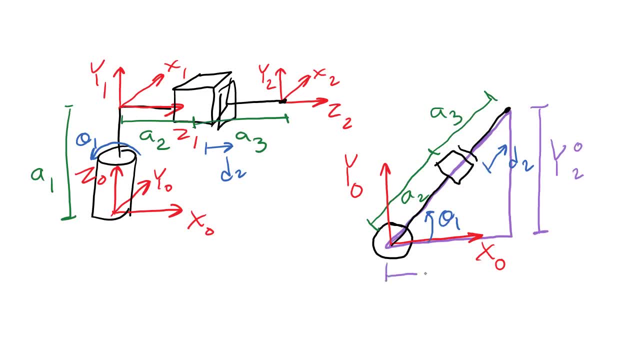 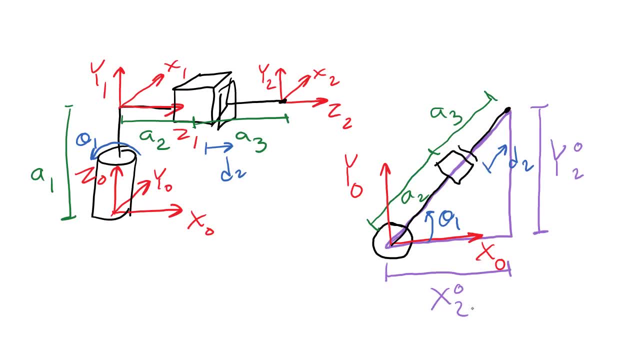 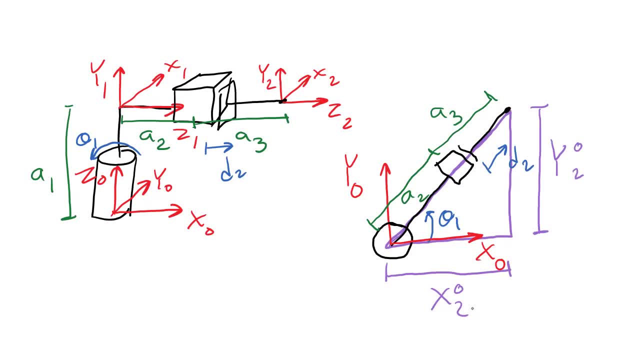 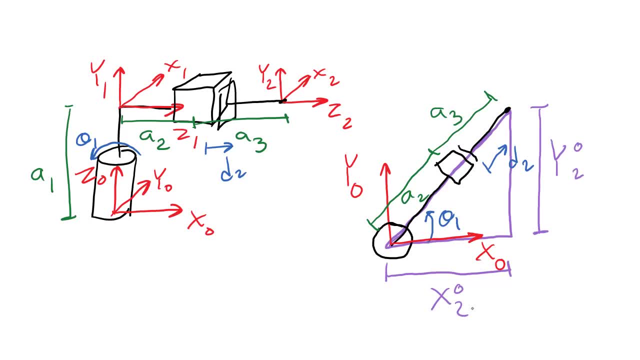 This distance here is x zero two, things that we know at the start of the problem. That's why this particular triangle is useful to us. We already know two of the sides: x zero two and y zero two. Next, I need to write. 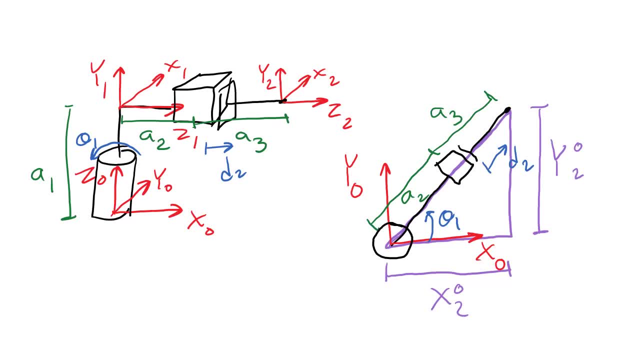 some triangle relationships to get some equations. There really are three kinds of triangle relationships that are going to be most useful to me. Number one is the Pythagorean theorem. Remember that the Pythagorean theorem is like this: If you have a right triangle and the two legs, 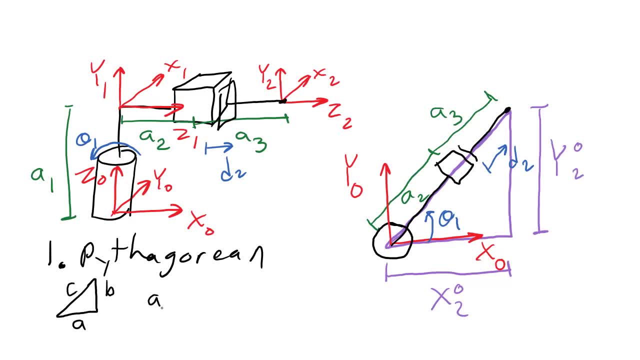 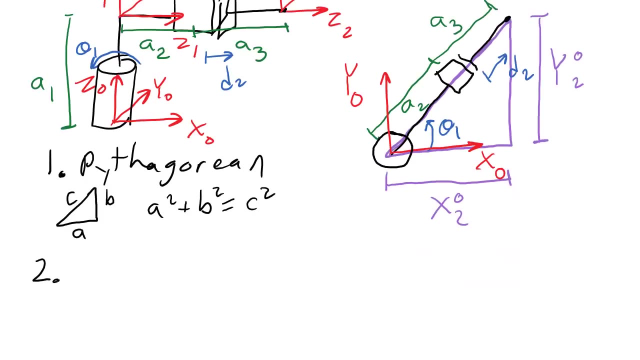 are called a and b and the hypotenuse is called c. this says a squared plus b squared is equal to c squared. The Pythagorean theorem only works if you have a right triangle. The second triangle relationship that will be useful is SOHCAHTOA. 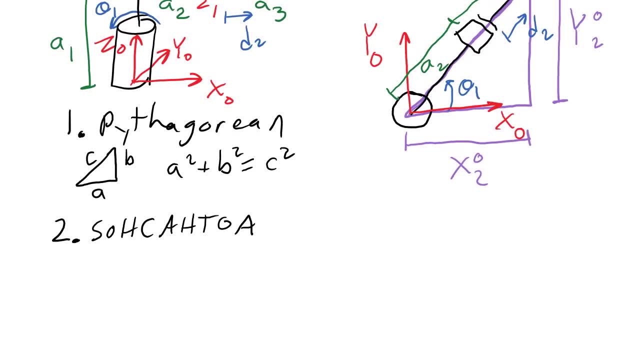 SOHCAHTOA. TOA is the acronym that many of us learned in high school or grade school. that helps us remember the sine, cosine and tangent relationships. For example, if we have a triangle like this and we call the sides A and B and this angle is theta, we know that the sine of theta 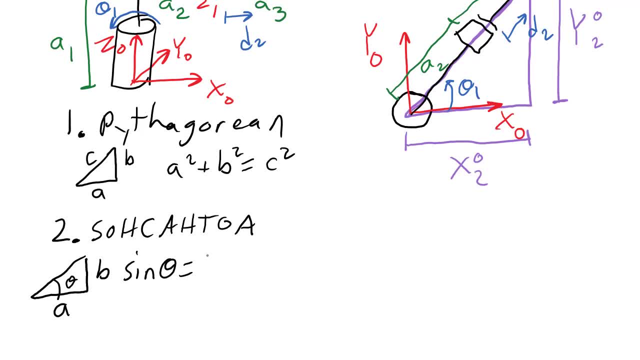 is the opposite over the hypotenuse. We'll call the hypotenuse C. The cosine of theta is the adjacent over the hypotenuse and the tangent of theta is the opposite over the adjacent. These two things both work only if we have a triangle like this. 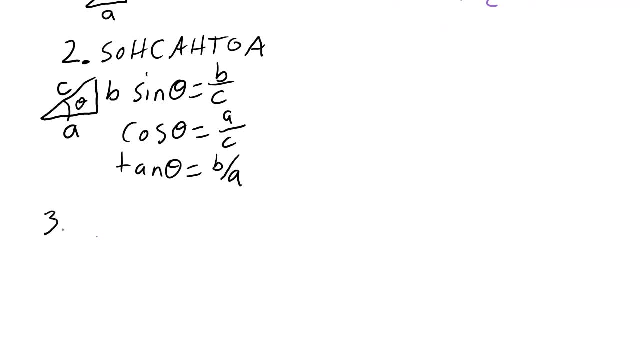 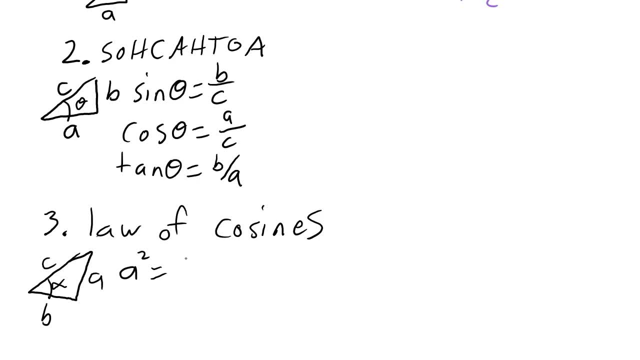 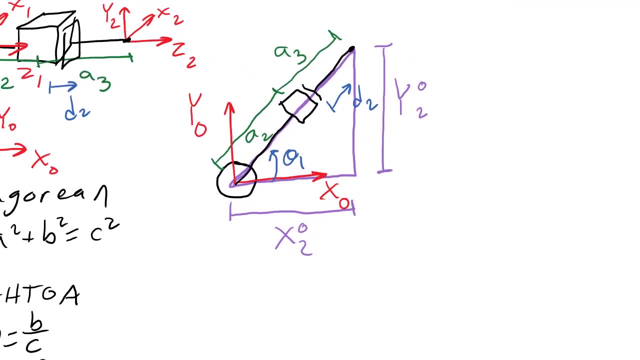 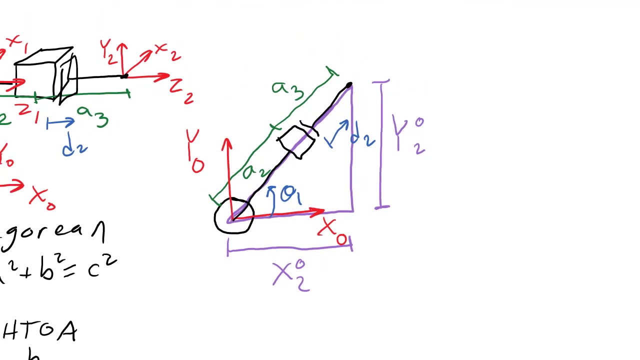 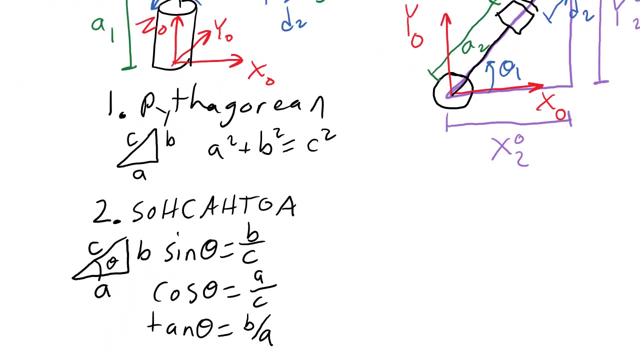 cosines says that a squared is equal to b squared plus c squared minus 2 bc cosine alpha. Now back at this example we're working through. which triangle relationship among the three that we have available to us should we use? Well, we have a right triangle, so we can use one or two. 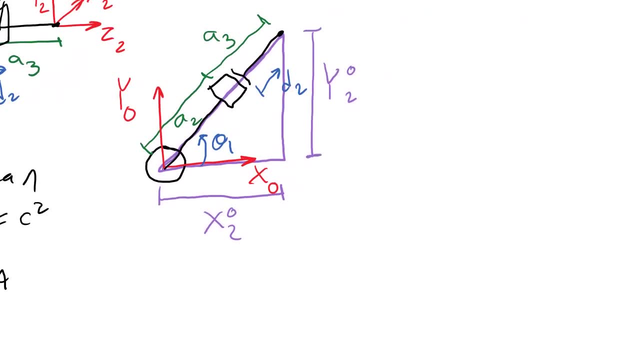 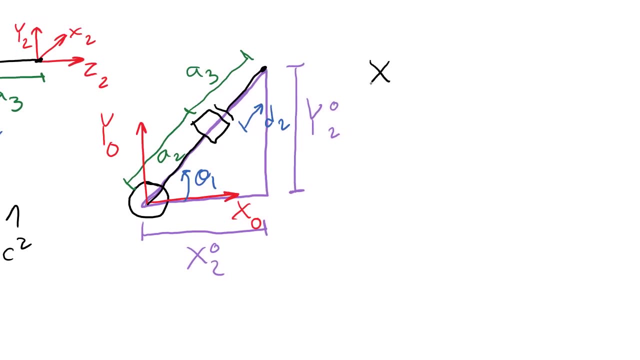 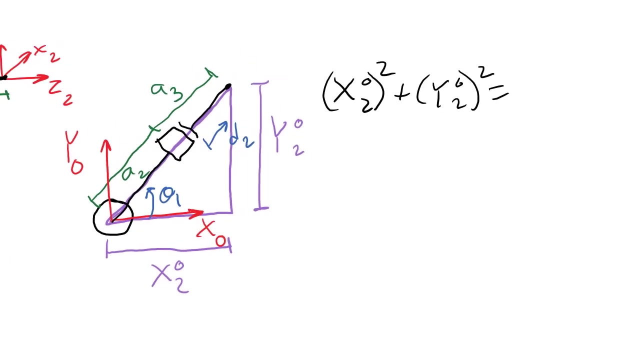 in addition to three. Let's start by using the Pythagorean theorem. So x 0, 2 squared plus y 0, 2 squared is equal to the length of the hypotenuse squared. What is the length of this hypotenuse? 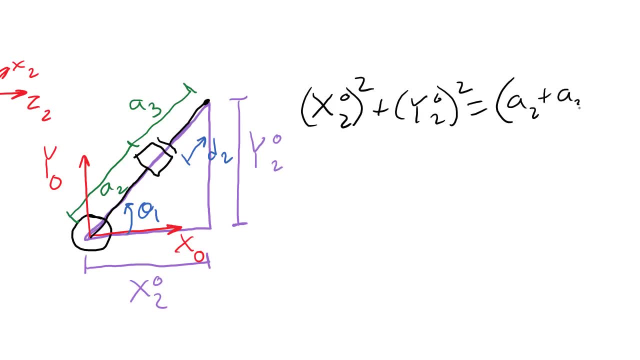 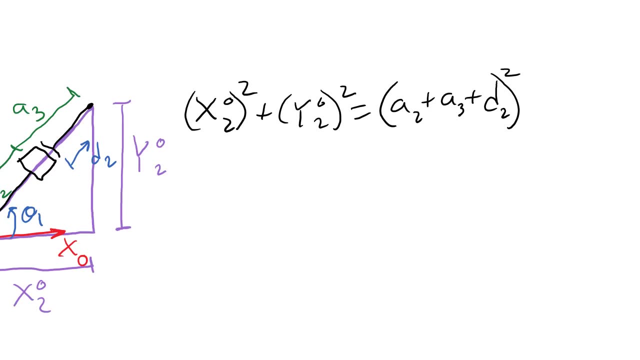 The hypotenuse length is a 2 plus a 3 plus d 2 squared. Now, in inverse kinematics, we're trying to have x and y be the input and we want to solve for the joint variables, which in this equation is d 2.. 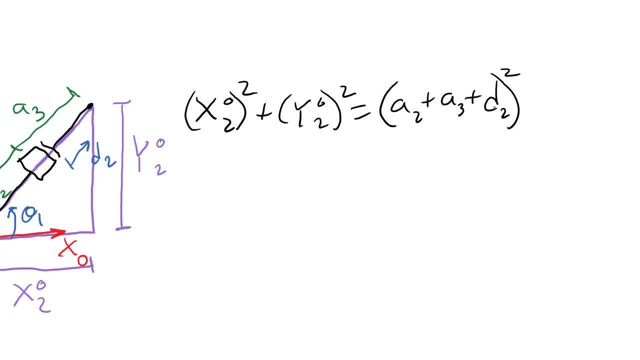 So we're going to solve for the joint variables, which in this equation is d 2.. So we're going to solve for the joint variables, which in this equation is d 2.. So I need to rearrange this equation a little bit to solve this for d 2.. 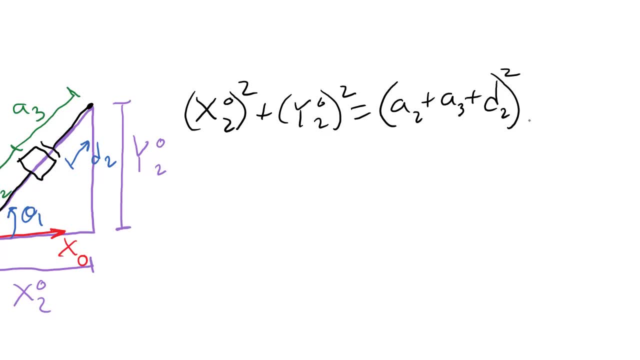 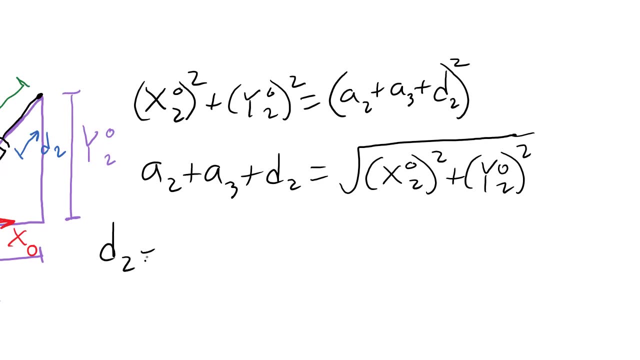 I'll start by square rooting both sides. Now I'll solve for d 2 by subtracting a 2 and a 3 from both sides. Now I have a joint variable on the left and on the right. I have only things that I know. 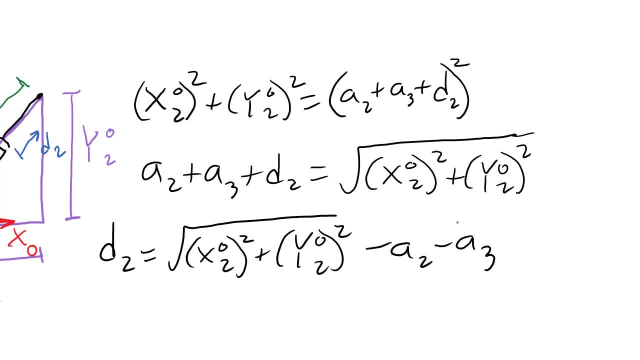 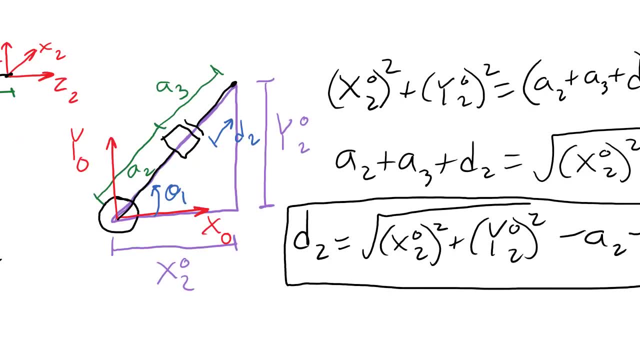 The values of the link lengths and our input, x and y. So I'm done with this equation. Now, I'm not done with the problem yet, because I still need an equation for theta 1.. To get an equation for theta 1, let's use SOHCAHTOA. 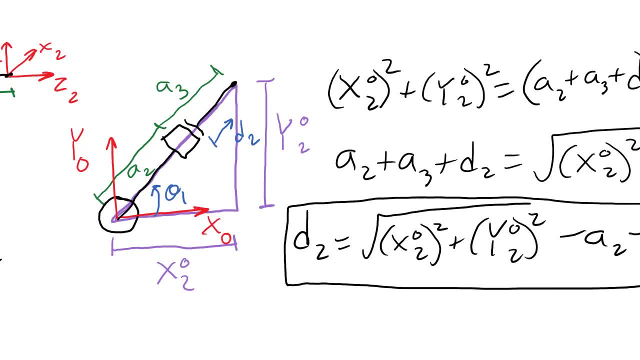 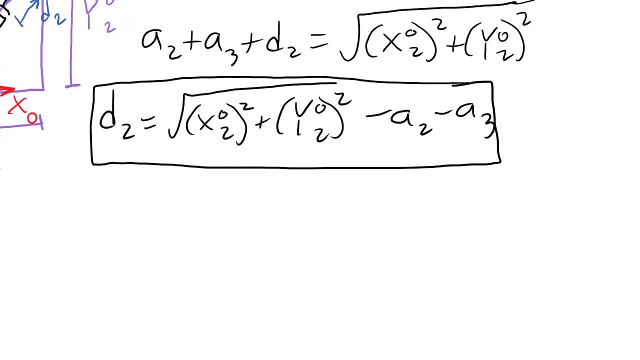 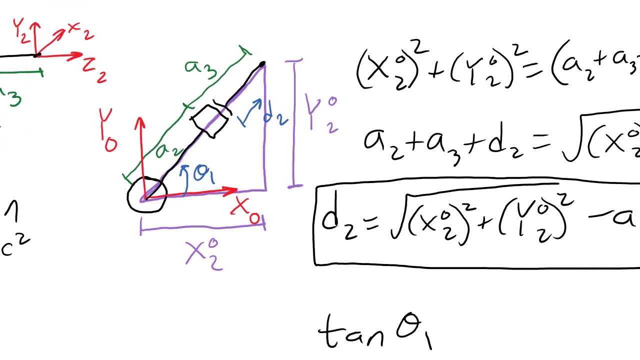 When we're using SOHCAHTOA. anytime I can use the tangent, my solution will end up being more robust than in other cases, So I'll write this equation: The tangent of theta 1 is equal to opposite over adjacent, y over x. 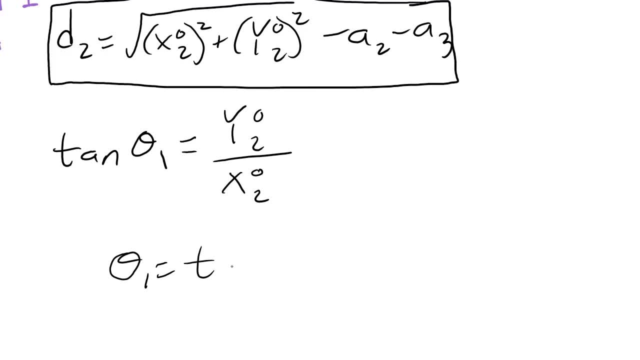 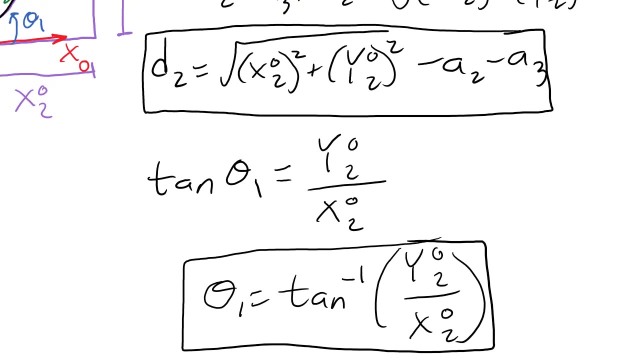 And now I'll solve for theta 1. I have a joint variable on the left and on the right. I have only things that I know, So this equation is finished. Also, I'm finished with the whole problem because now I have one equation for each joint. 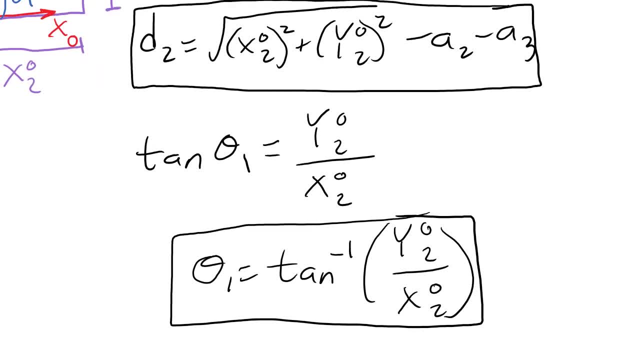 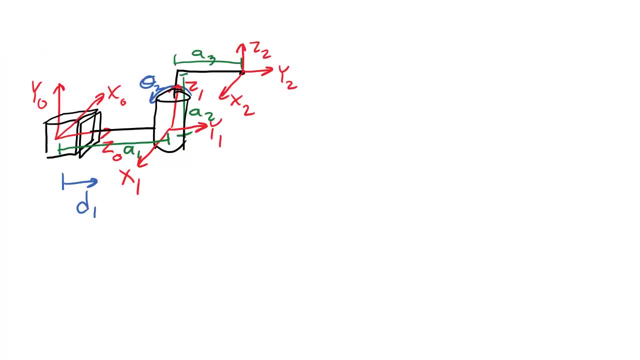 So now I have one equation for each joint variable. Let's do one more easier example before we go back and do a hard one. Okay, let's do inverse kinematics for THIS manipulator. This manipulator starts with a prismatic joint and then has a revolute joint attached to it. 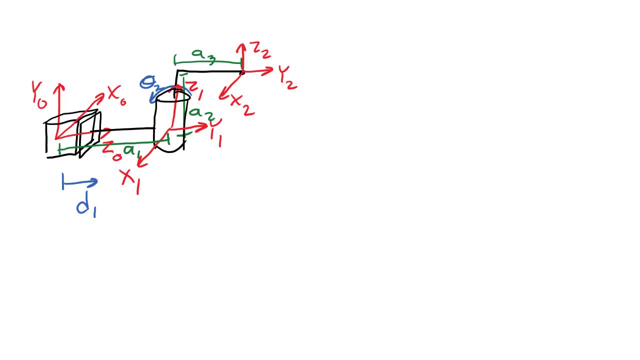 Let's start by drawing this manipulator from the top down view. From the top-down view, The first stop is the manipulator. first joint will look like a square, Then we'll have a circle for the second joint and then, when I show the last link, I'm going to draw it as though theta 2 was 45 degrees. 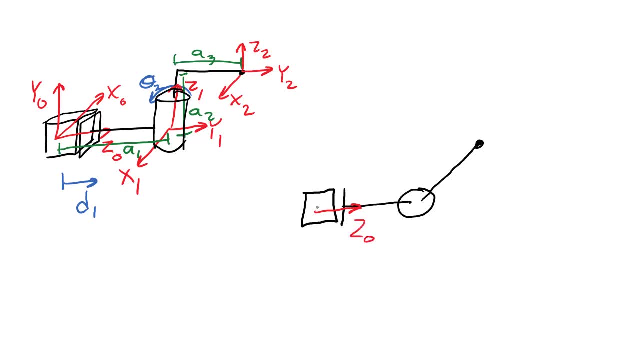 In this picture. this is the z zero axis and this will be the x zero axis. We can't see y zero in this picture because y zero is pointing straight up at our eyes. We're looking down at this manipulator. The joint variable d1 is here and the joint variable theta 2 is. 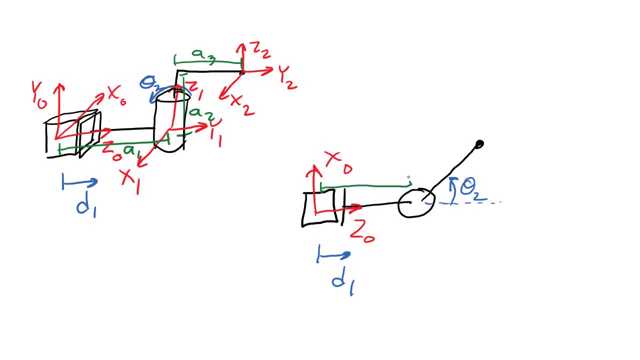 right here. This is the length a1, and this is the link length a3.. Okay, now the first thing we need to do is identify the end effector position. in this picture, The end effector is right here, so now I'm going to make a triangle that shows its position. 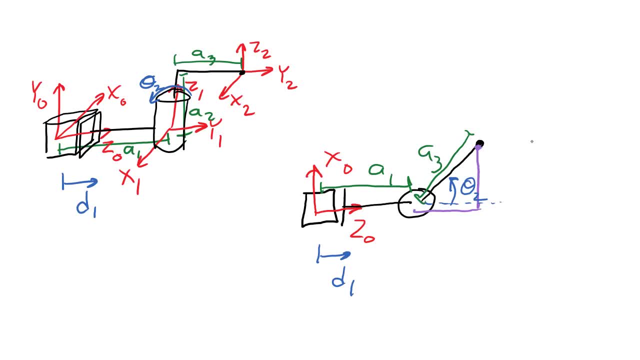 It's tempting to use a triangle to make a triangle. We can use the link length a3 as the hypotenuse here, but that isn't true if we're trying to show the position of the end effector. The zero. zero position is all the way back. 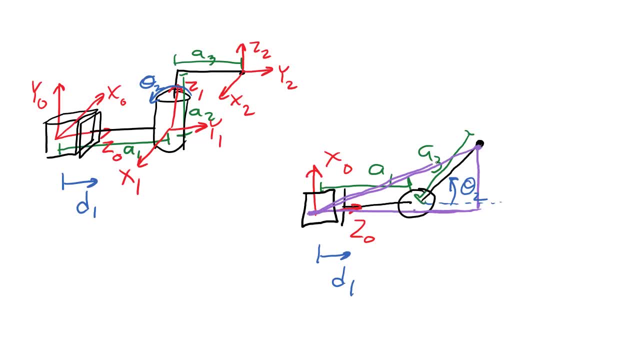 here, and so the triangle that shows the position of the end effector is this triangle. This distance here is the x position of the end effector in the base frame, and this distance here is the x position of the end effector in the base frame. This distance here is the. 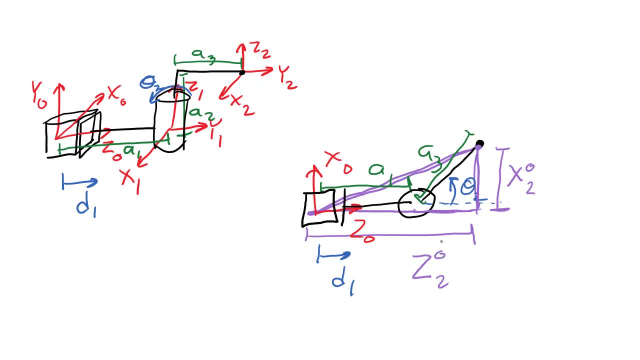 z, position of the end effector in the base frame. Now, using this triangle and any other triangle relationships that we need to draw in, we need to find some relationships that say d1 equals something, where this something only includes things we know on the right hand side. and we need another equation that says: 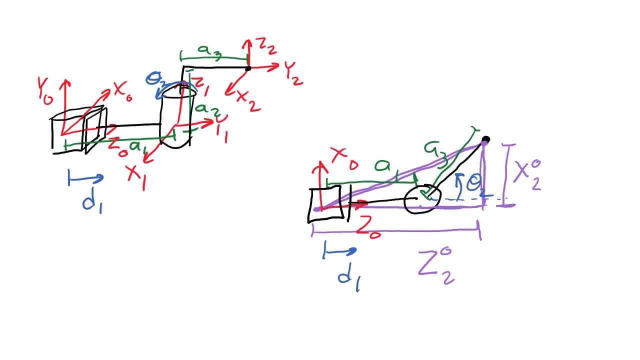 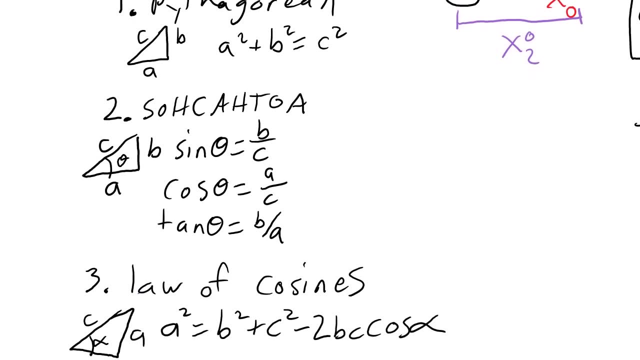 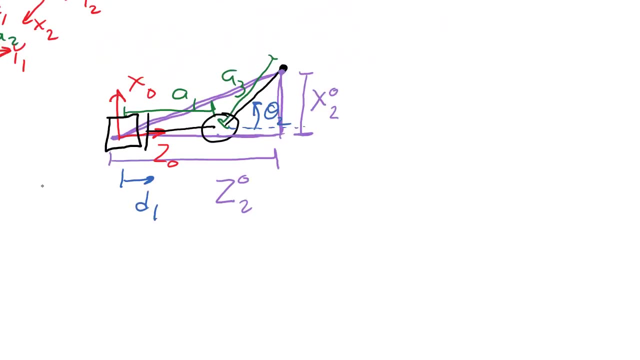 theta 2 equals something. Remember theta 2 equals something. Remember that we have three options at our disposal. We have the Pythagorean Theorem, SOHCAHTOA and the Law of Cosines, Sometimes the one triangle that shows the position of 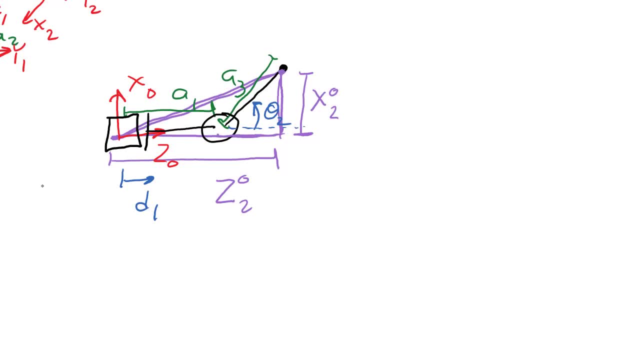 the end effector isn't enough to get us all the way where we need to be, and we need some other triangles. The next triangle that we're also going to use is this triangle. here We're just putting everything in the shape corner. Say, angle is equal to therizon of the 180 degrees. 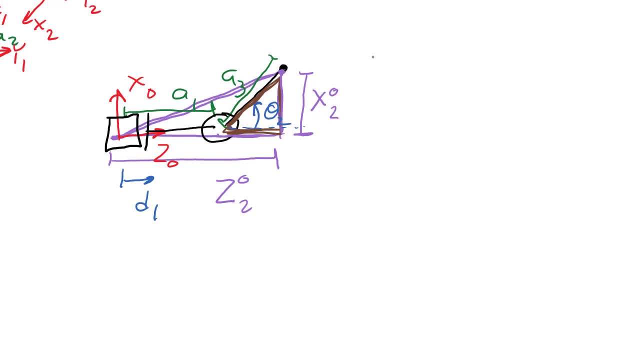 so to easily find it, we need the angle of the angle from the dx 0 to half cross x, as well as the angle of the angle of the angle, or to use the Campbell formula, We're using it as the turbulent Initiative, now that we're using it to calculate 0 plus. 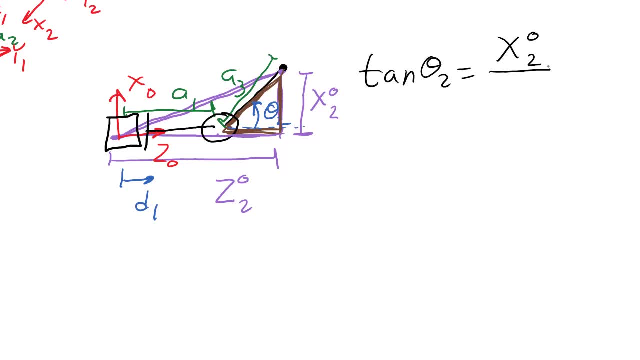 minus And now using the 34-圈 rectangle for the angle we're using, we're going to notice that it's actually going to lose some little thing if we use the riding angle as a contradiction. But here I have this X icon on the edge here which I actually love to calculate focus. 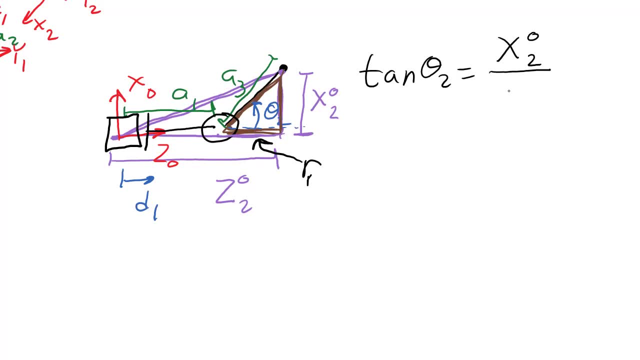 and adding space to the angle, so that when I add space I don't have to add the region again divided by r1.. How could we find a value for r1? We could use the Pythagorean theorem. We could say that r1 squared plus x02 squared is equal to the hypotenuse squared. And here 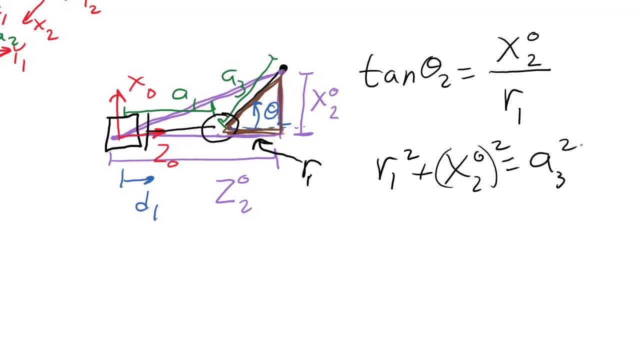 the hypotenuse of the brown triangle is a3.. I'm going to solve this equation for r1.. I'm going to label this equation 1.. Then I'll solve the tangent equation for theta2.. And I'll call this equation 2.. Numbering these equations can help us keep track of what order. 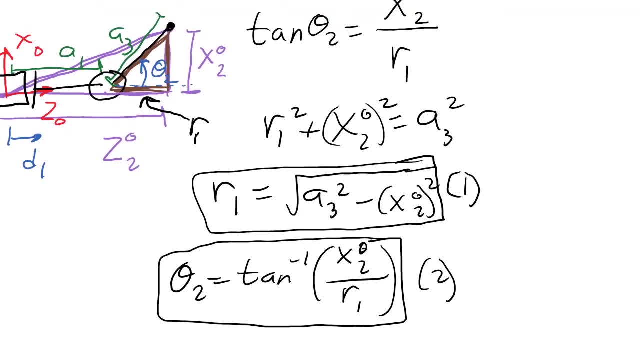 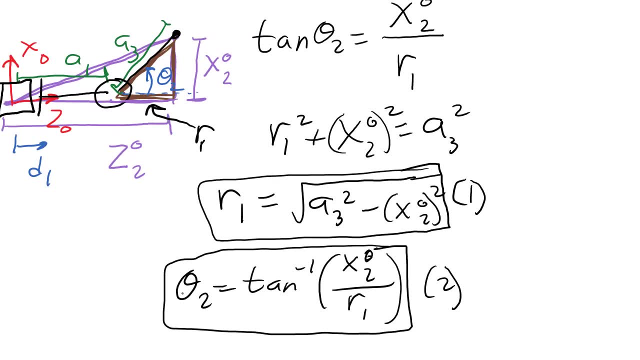 we need to put these equations into our code. For example, we can start by solving for r1 in our code. Then we'll have a value for r1.. Then we can plug into equation 2 to solve for theta2.. But of course we couldn't do this. the. 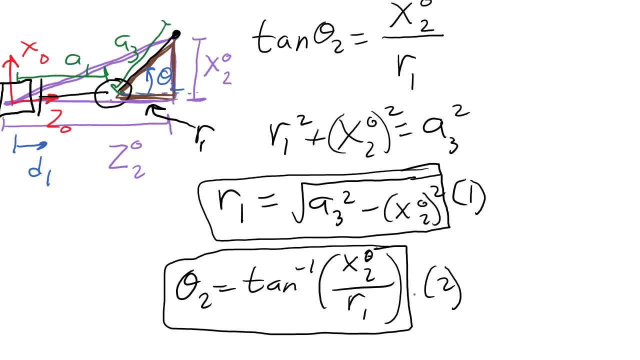 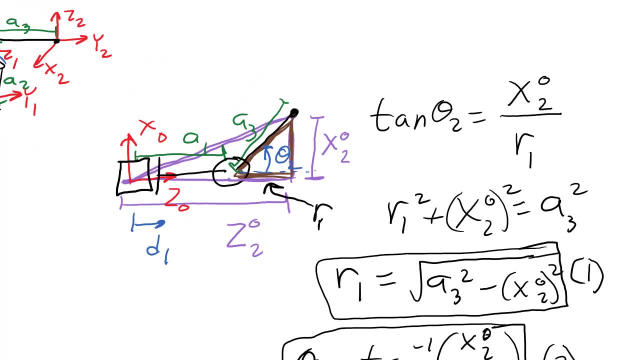 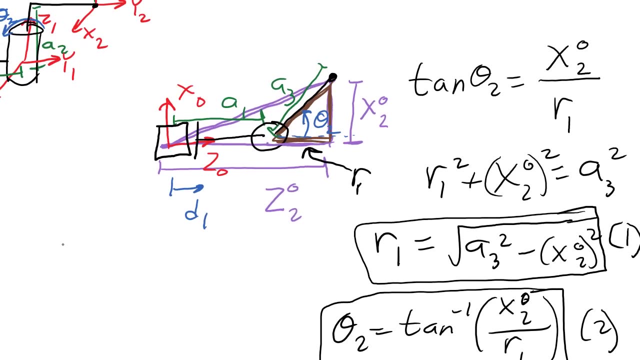 other way around. If we try to solve for theta2 first, we won't have a value for r1.. All right, I still need an equation for d1.. To get d1, let's try writing an equation like this: z02.. 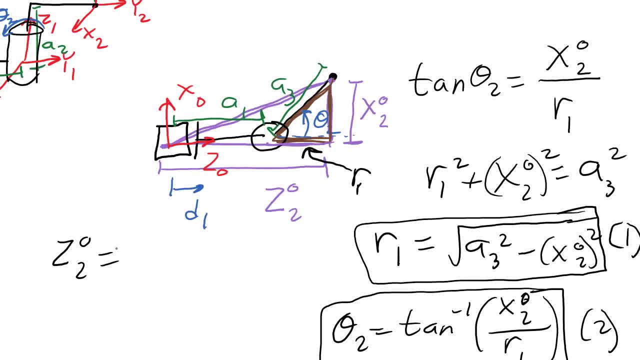 That is, the entire distance of the bottom of the purple triangle is equal to a1 plus d1.. That's the distance from the first joint to the second joint Plus r1.. Now I'll solve this equation for d1.. 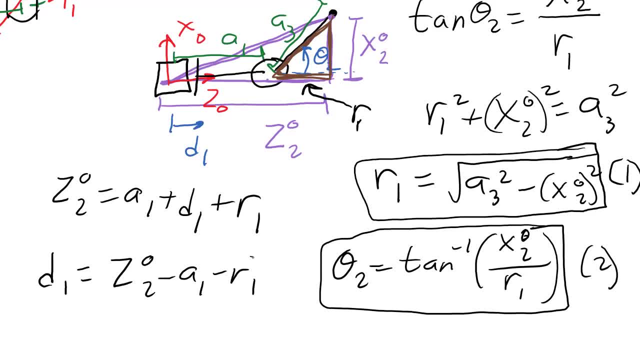 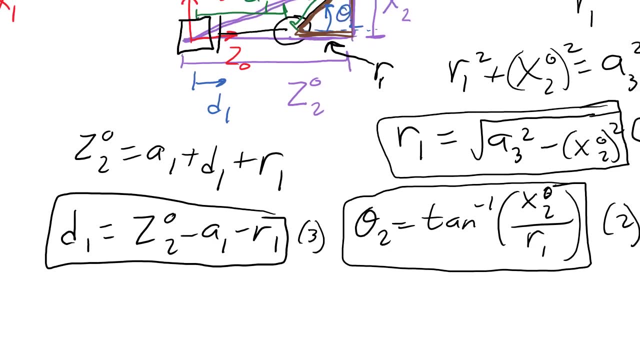 Since we've already found the value for r1 in equation 1,, I can stop here and call this equation equation 3.. When I put this into my code, as long as I put these equations in this order: 1,, 2,, 3,- 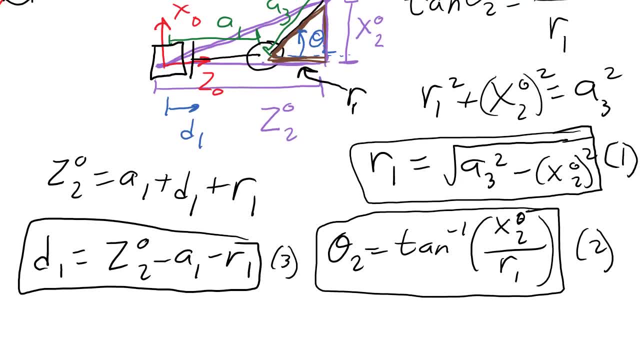 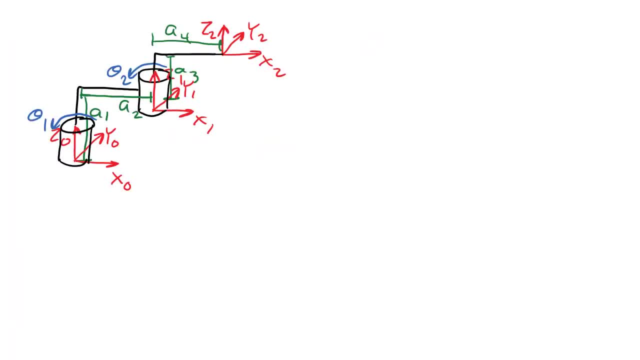 we'll be able to solve for theta2 and d1, given the values of the link lengths and the position of the end effector only. Okay, are you ready for a more difficult example? Here's the kinematic diagram for the manipulator that we have built on our board. 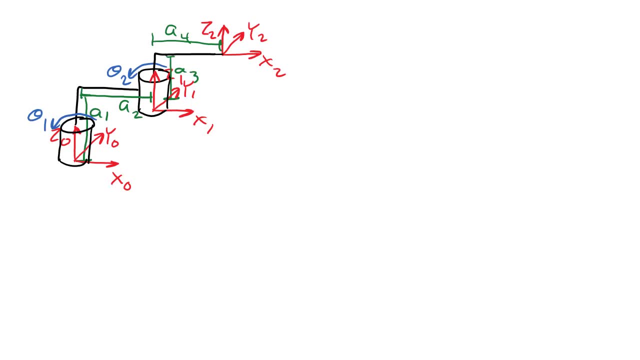 Z02.. If we can find the inverse kinematics equations here, we can go and put these equations into our PSOC code and see if we can actually position the end effector where we want it. Let's start by drawing this kinematic diagram from the top-down view. 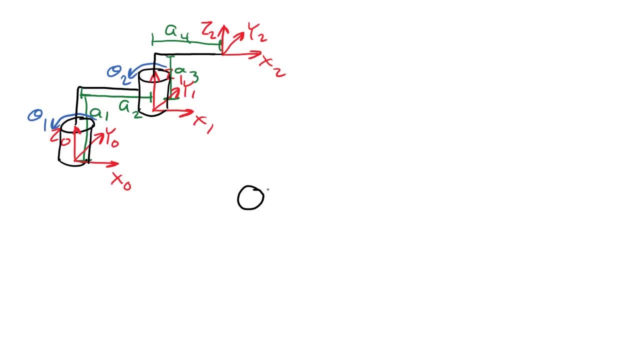 The first joint will look just like a circle. Then I want to draw theta1 at a 45-degree angle. Then we have the second joint, also looking like a circle. Now I'll draw the next link, for theta2 also being not zero. 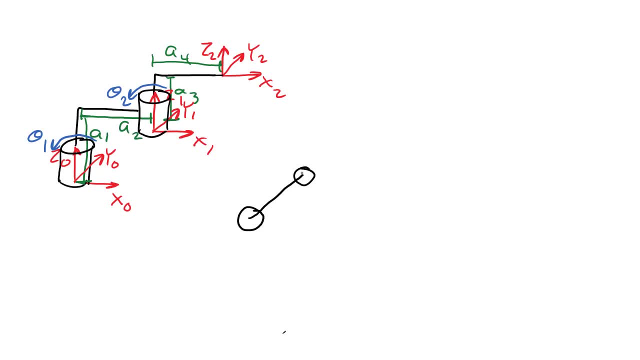 But I'm not going to quite draw it at 45 degrees, otherwise the link will be going straight up and that will make it hard for me to see. So I'm going to draw it like this instead. This is the x0 direction. This is the x0 direction. 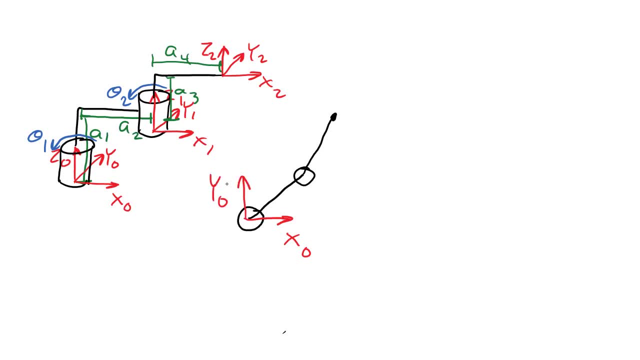 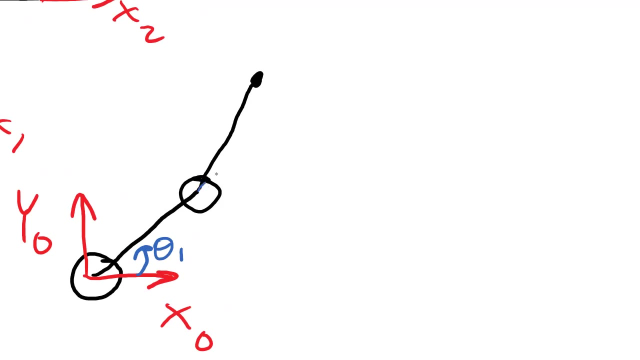 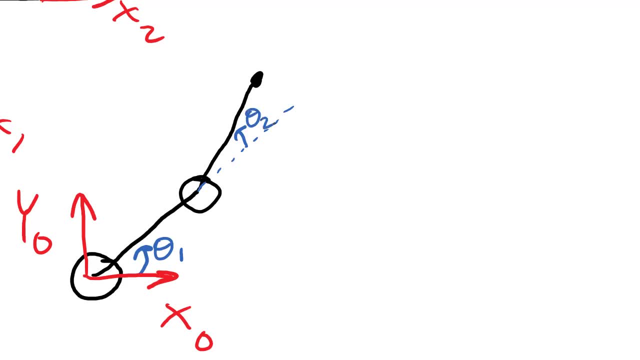 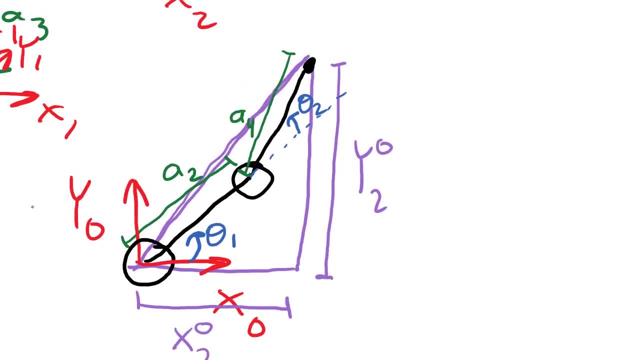 And this position here is the x position of the end effector in the base frame. And this position here is the x position of the end effector in the base frame. the end effector in the base frame, The other triangle that will help me solve this problem. 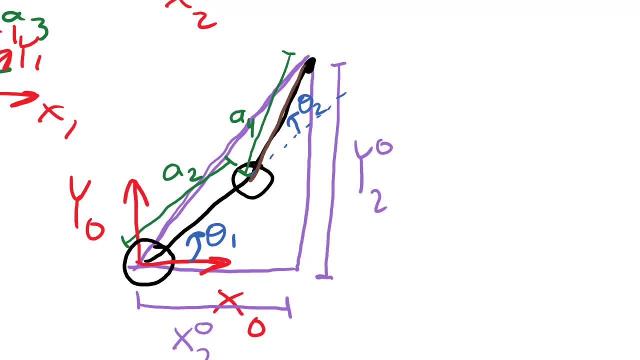 I'm going to draw in brown. That triangle is this one: The purple triangle is a right triangle and the brown triangle is not a right triangle. Remember that there are two triangle relationships. I can use for right triangles the Pythagorean theorem. 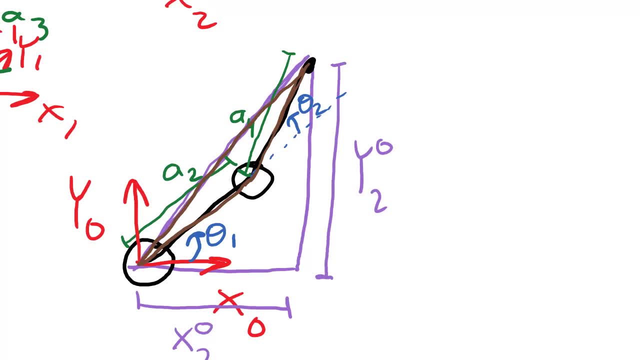 and SOHCAHTOA and one triangle relationship, the law of cosines- that I can use on triangles that are not right triangles. Let's start by using the Pythagorean theorem: The length of this side, which is overlapping between the two. 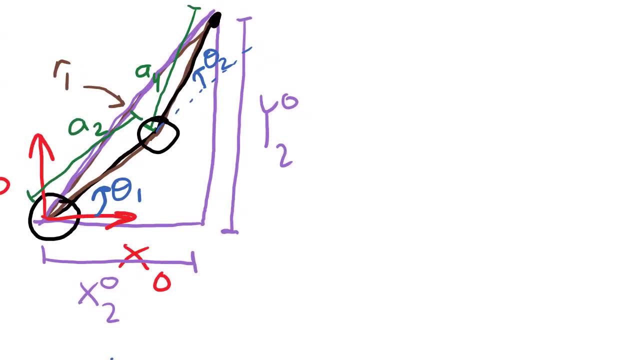 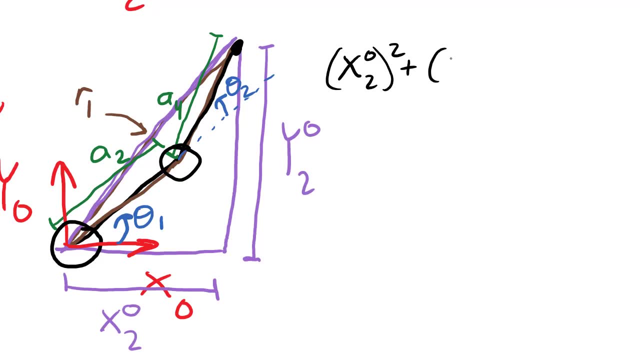 triangles. I'm going to call r1.. We'll solve for the length, The length of that side, by going x02 squared plus y02 squared is equal to r1 squared, And then I'll solve for r1.. I'll call this equation equation 1.. 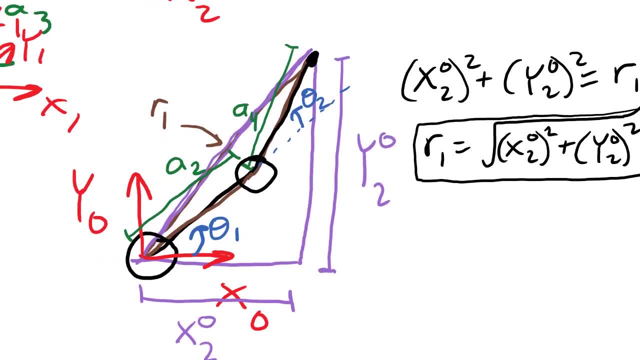 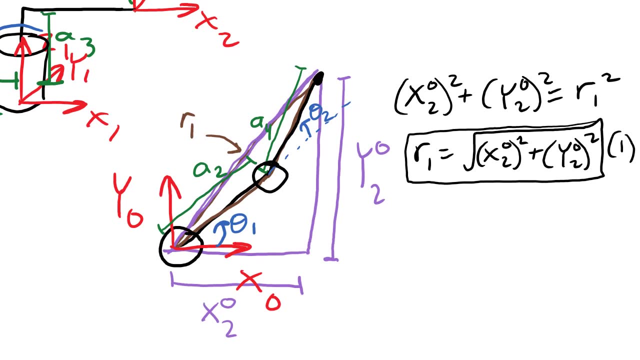 Now that I know the value of r1, let's look back at the brown triangle, the one that is not a right triangle. In that triangle, I know the lengths of all three sides And because of that I can use the law of cosines. 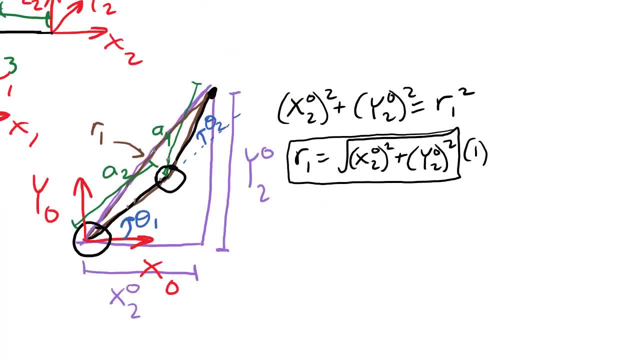 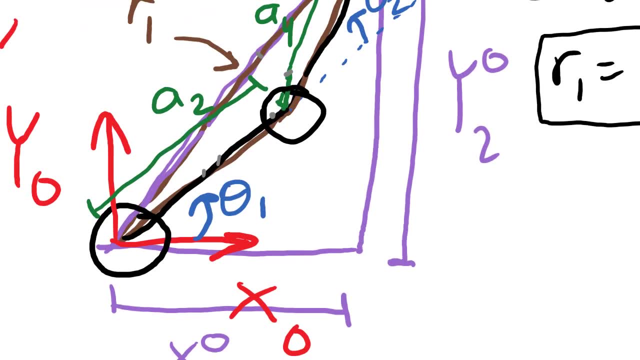 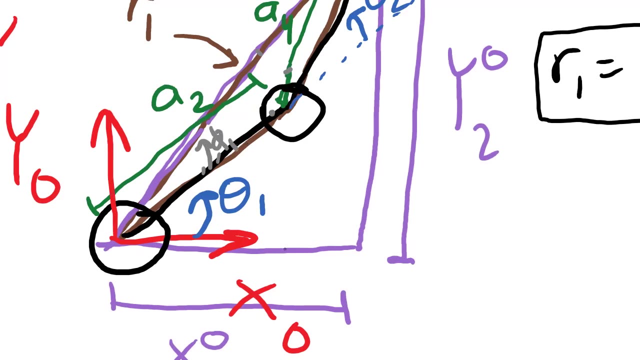 to find the values of angles. In order to make use of the law of cosines, I need to label a couple new angles. Let's call this angle right here v1.. Let's call this entire angle in the purple triangle v1.. 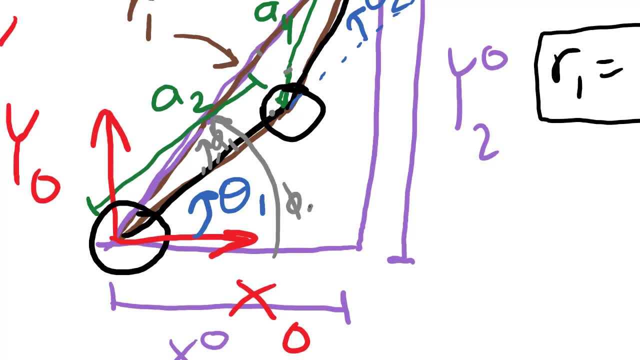 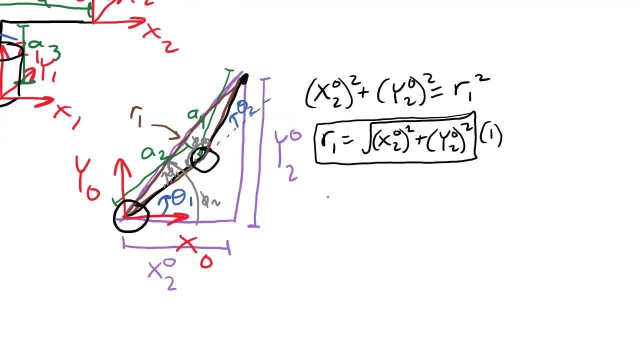 Now I can use v1 and v2 to write a relationship with theta 1, like this: theta 1 is equal to v2 minus v1.. If I can get expressions for v1 and v2, I can find theta 1.. 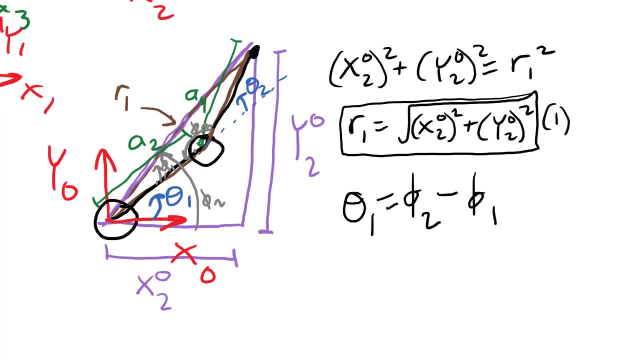 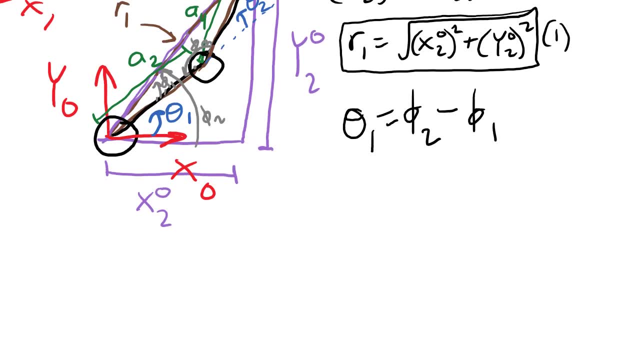 Let's start by getting v2 from the purple triangle, using it to find theta 1.. Let's start by getting v2 from the purple triangle, using it to find theta 1.. Let's start by getting v2 from the purple triangle. 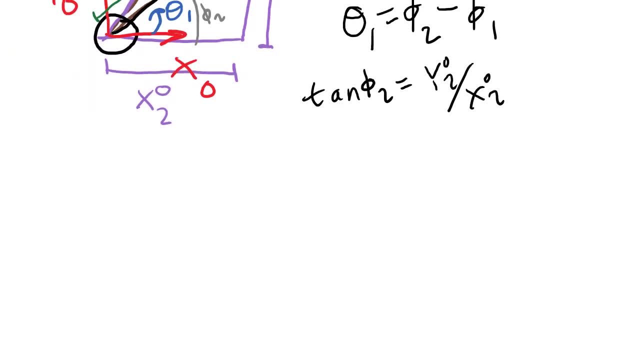 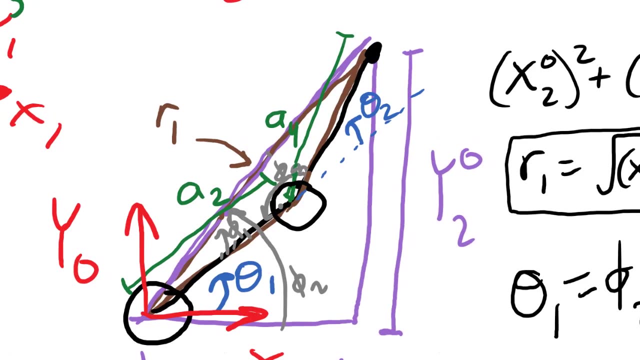 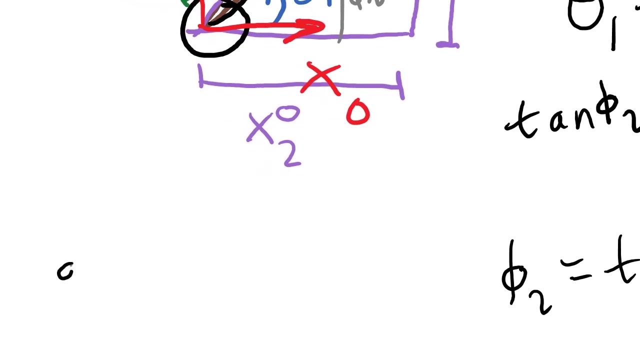 using it to find theta 1.. And then I'll solve this equation for v2.. Next, we want to get v1. v1 is inside the brown triangle And a4 is the side that is across from v1. So we can use the law of cosines to get v1, like this: We start with the side across from the angle v1, and v2.. Let's start with the side across from the angle v1, and v2.. Let's start with the side across from the angle v1, and v2.. 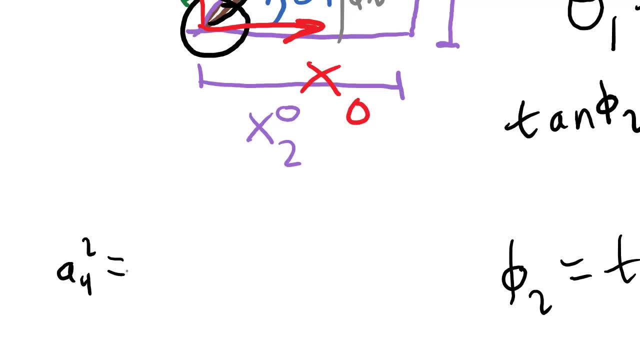 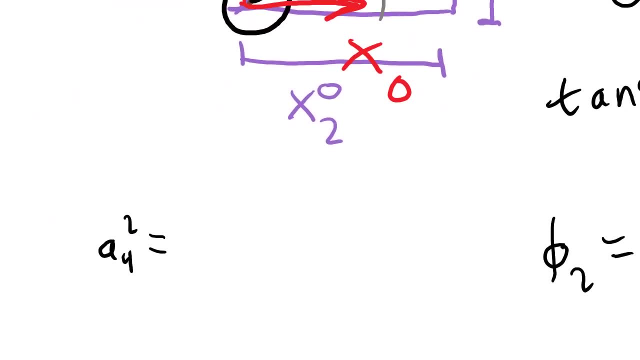 Let's start with the side across from the angle v2.. So we're againierzong the angle we're looking for. Then we square both of the other two sides, which in this case is r1 and a2.. Minus 2 times each of the other sides. 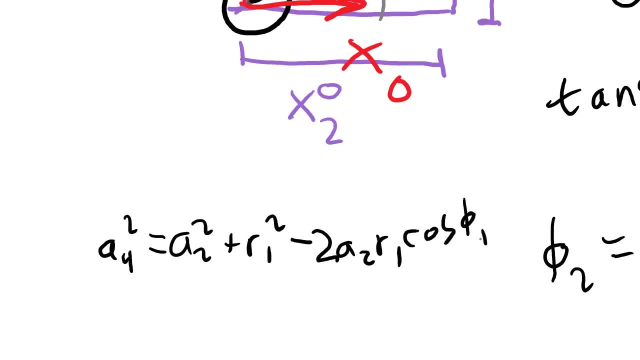 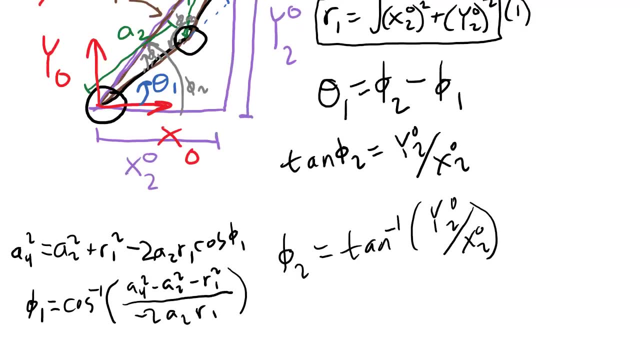 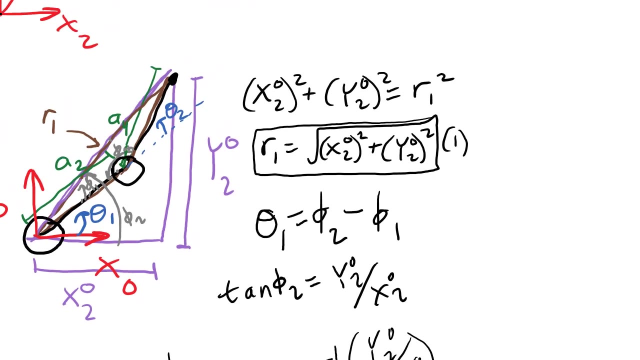 times the cosine of the angle that we're looking for, which is v1.. Now I just have to solve this equation for v1.. which is v1.. Now we can go back and number our equations. We've already solved for r1.. 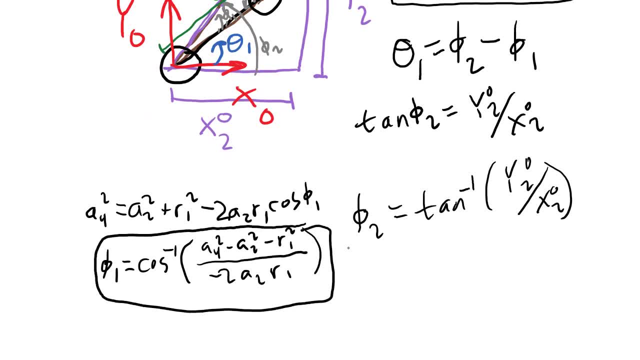 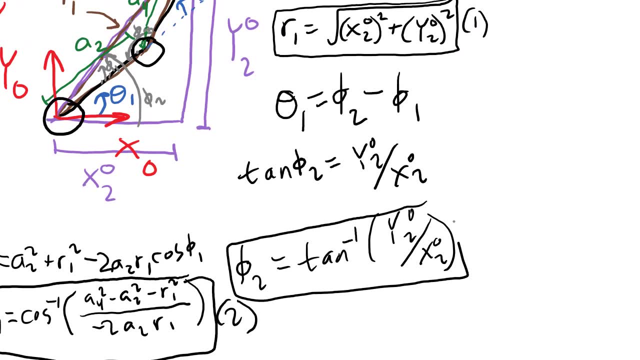 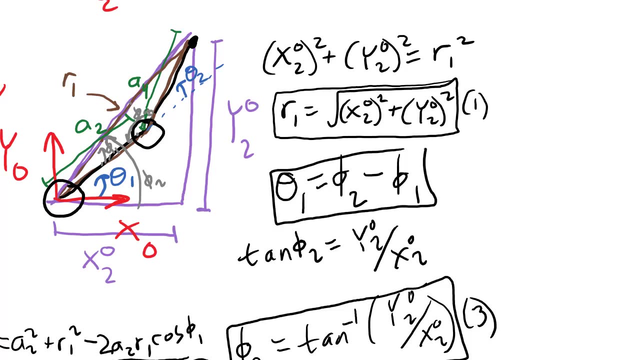 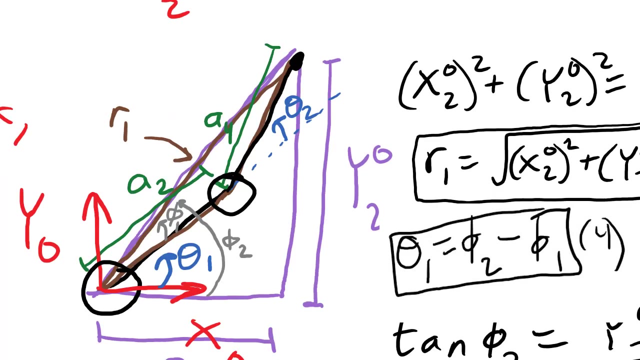 This will allow us to go and solve for phi1. And we can also solve for phi2.. Once we have phi1 and phi2, we can solve for theta1.. To find theta2, I need to mark one more important angle in this triangle. 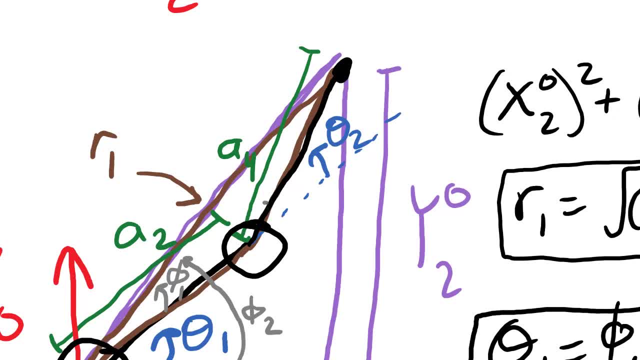 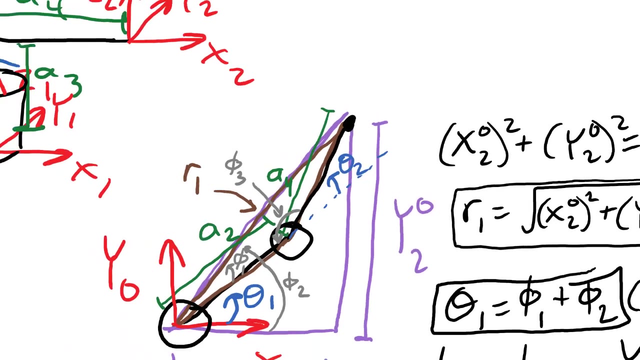 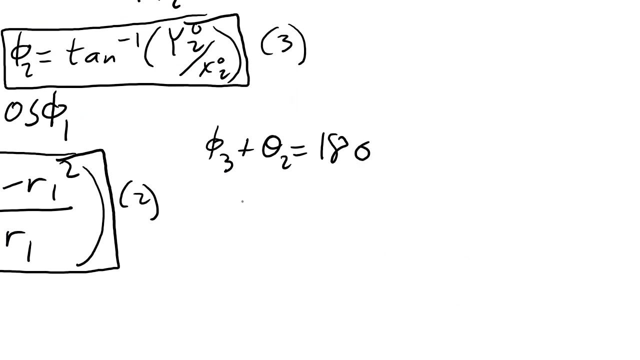 I'm going to zoom in and I'm going to call this angle right here phi3.. Now Notice that phi3 plus theta2 makes a line that is straight. So phi3 plus theta2 is 180 degrees. Let's write that down. 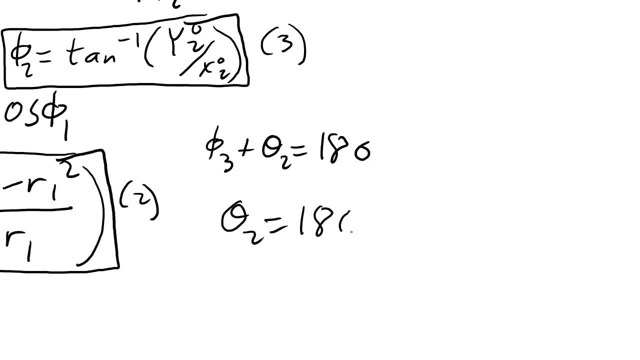 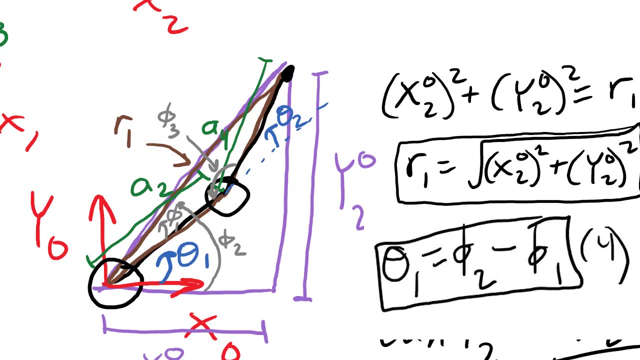 So we can say that theta2 is 180 minus phi3.. If we could find an expression for theta2.. For phi3, we would have theta2.. How could we get phi3?? Phi3 is one of the angles inside the brown triangle, which is not a right triangle. 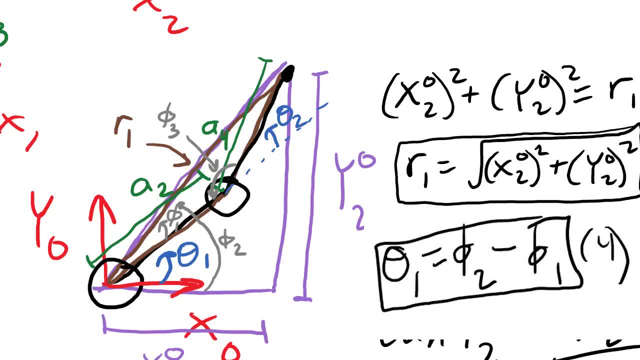 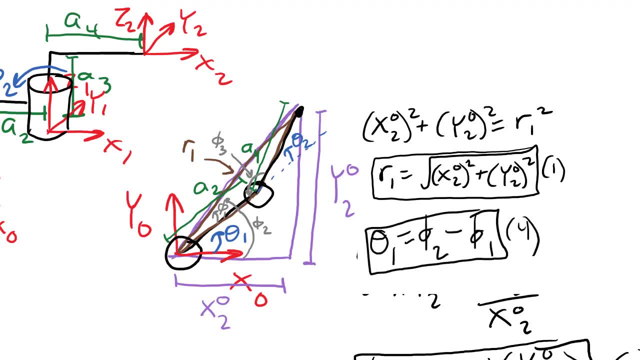 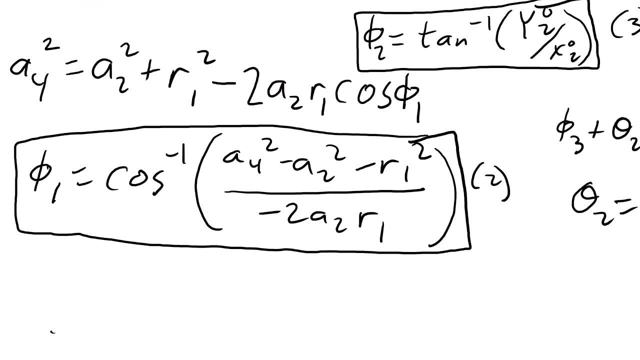 So we can use the law of cosines To use the law of cosines to get phi3, we'll start by finding the length of the line that is opposite phi3.. The length of the triangle side opposite phi3 is r1.. 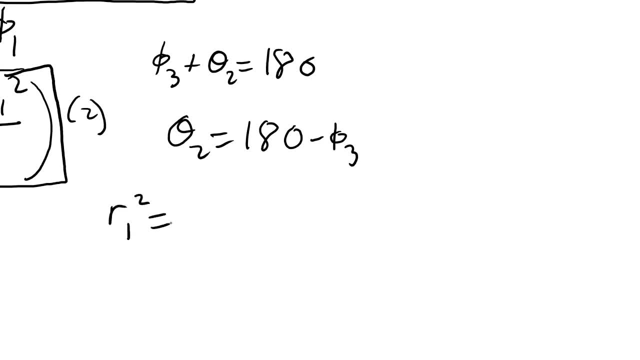 So we'll do. r1 squared is equal to. Now we need the lengths of the other two sides, a2 and a4. So a1! A2 squared plus a4 squared, minus 2a2, a4 cosine. The angle we are looking for is b2.. 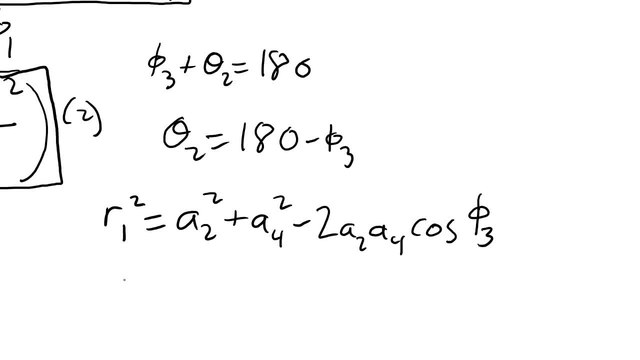 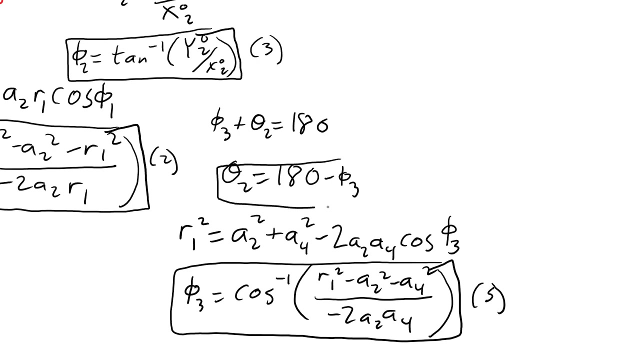 The angle. we're looking for phi 3.. Let's solve this for phi 3.. Alright, the last equation that we numbered was equation 4.. So let's call this equation 5.. Finally, once we've found the value of phi 3,, we can use this equation 6, to find theta 2.. 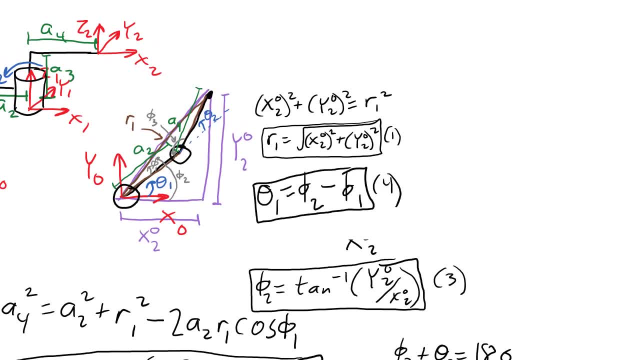 I know this was a lot of trigonometry and algebra to get these equations. Don't worry if you don't think you could do this on your own yet. We'll practice this a bunch both in Robotics 1 and in Robotics 2, until you feel comfortable with it. 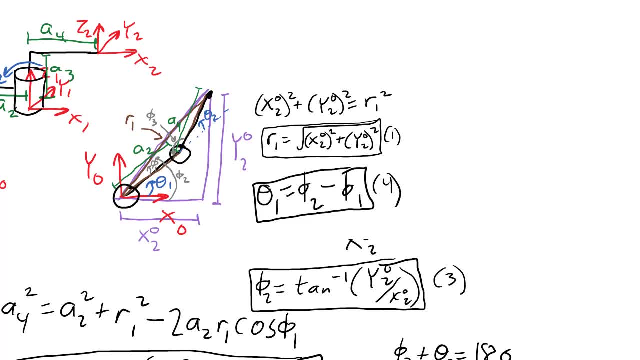 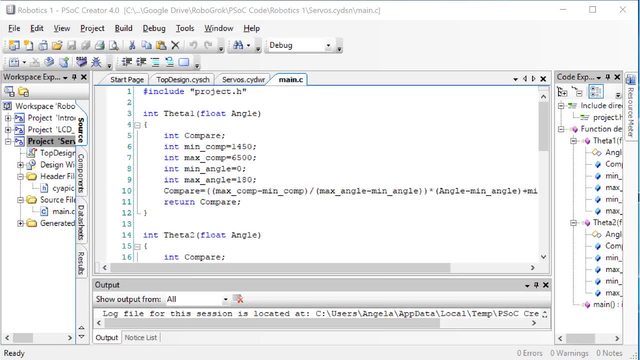 Right now we're going to take these equations and solve them for phi 3.. We're going to put these equations into our code and I'm going to show you how to use these equations to position the end effector. Start by opening PSoC Creator and open up the project that we were working with last time. 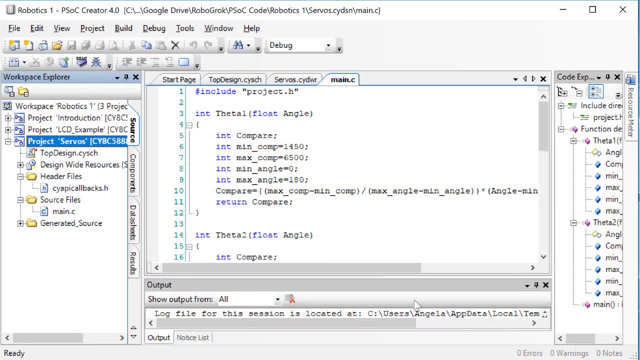 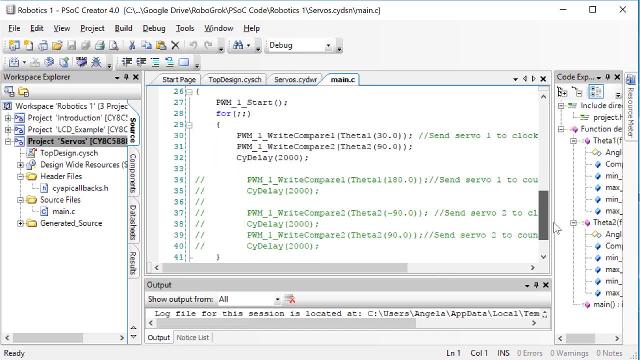 Remember that this project is called Servos. The C code in the Servos project simply sets two angles. That's still what we want to do, except now. we want to use our inverse kinematics equations to calculate which angles these should be given a desired x, y position of the end effector. 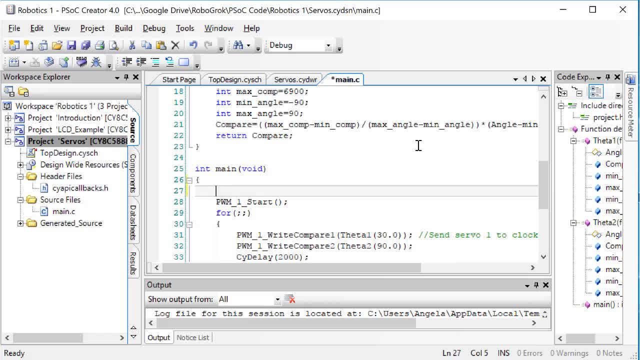 Go up to the beginning of main and let's create two variables to serve as input where we want the end effector to be. Let's just call them x and y. For now let's just set them equal to 1.. We'll go back and change them after we finish writing our code. 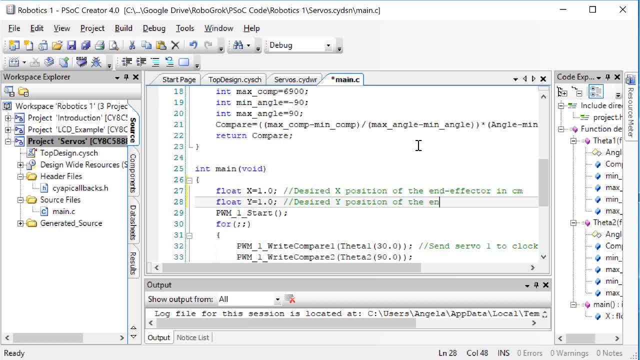 We'll make these two variables floats so that we could give them decimal points, if we want to. Now we want to enter the equations that we derived previously. We need to start with equation 1, and work through to the last equation, which for us is equation 6.. 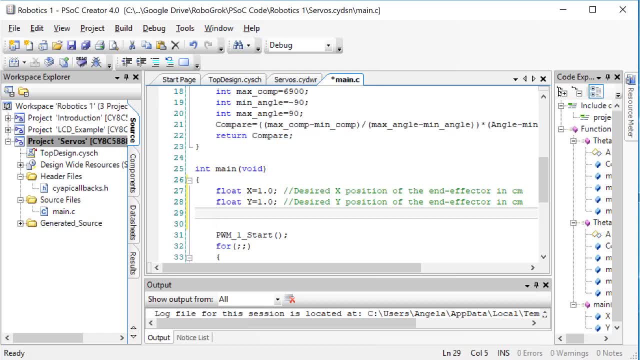 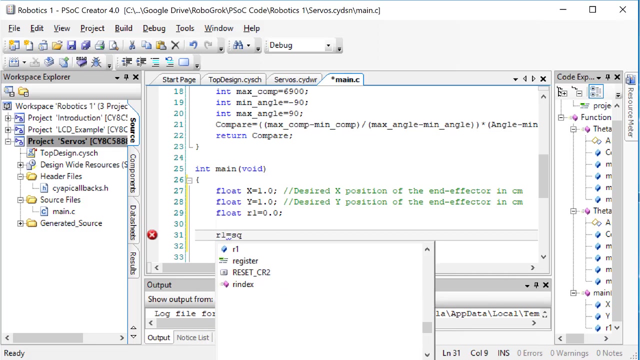 Equation number 1 calculates the value of R1, so we need to create a variable to hold R1.. Now let's go ahead and calculate it. Our equation says that R1 is equal to the square root of x squared. Our equation says that R1 is equal to the square root of x squared. 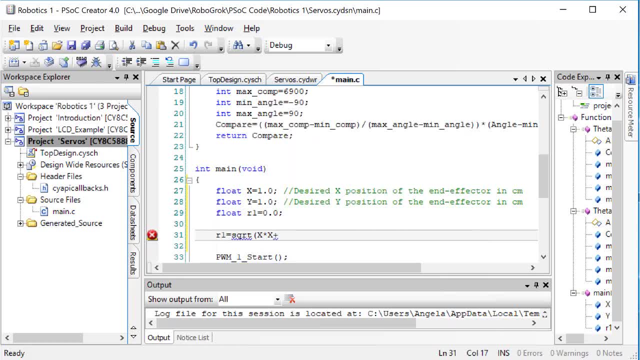 That's going to be minus 2.. That's going to be minus 2.. That's going to be minus 2.. just do x times x plus y, squared y times y. Now you'll notice that we get a warning here. It says that we've implicitly declared the library function. 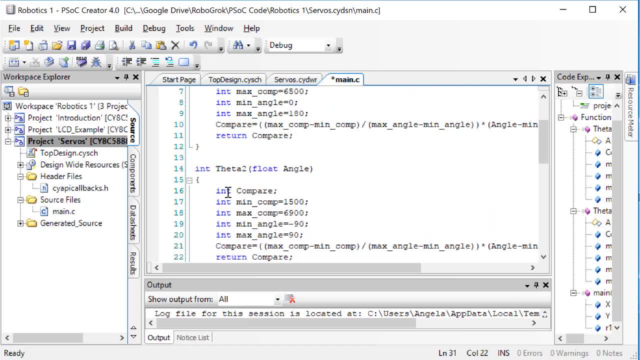 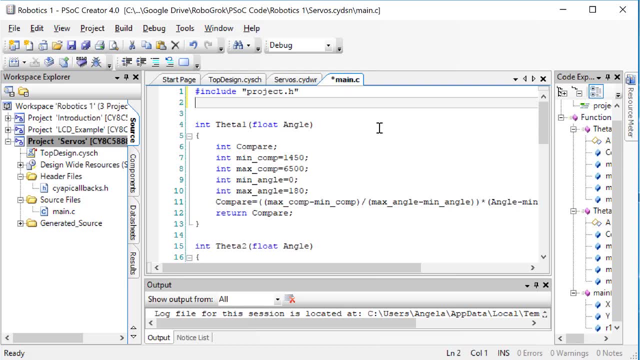 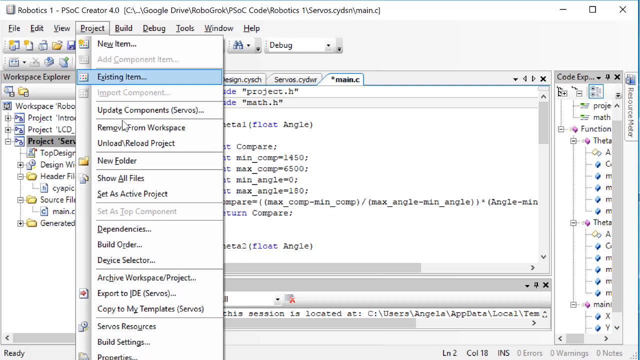 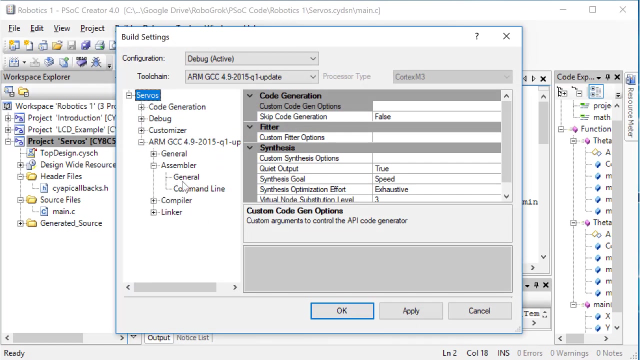 square root. Square root is not a function that is included in project dot H. It's included in another library called Math. So up here we need to do include math dot H. then we also need to go to project build settings and in the 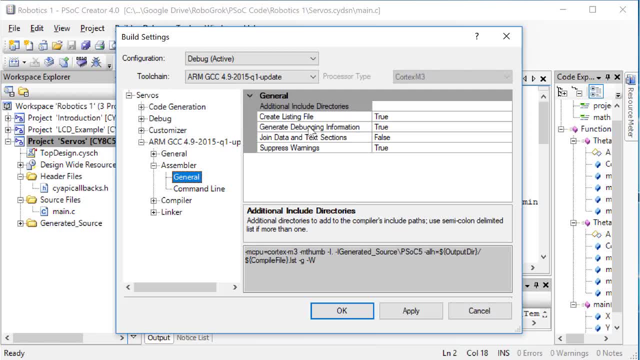 assembler, click on general and then where it says additional inclu- cluduron. Also on that new folder there is a white note button called h. If the water andал 마 세�ена, directories type M and hit enter. M stands for math, we need to do this also. 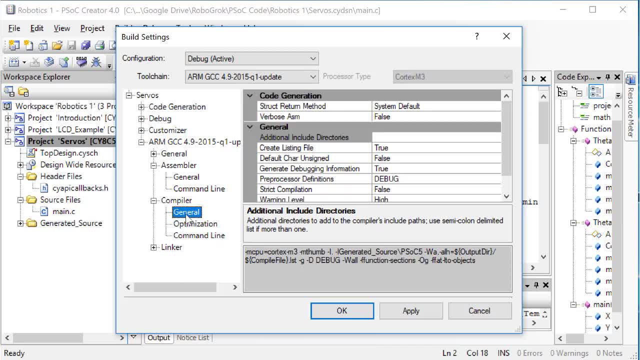 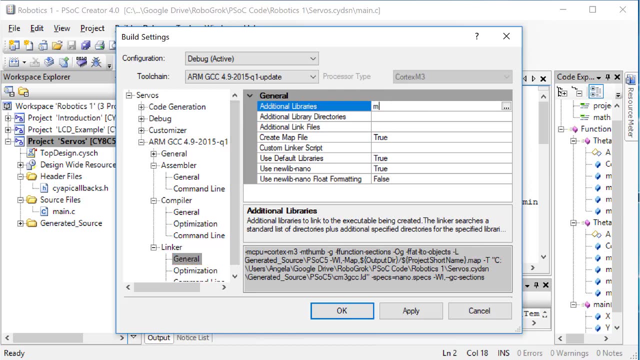 in the compiler. so go to compiler general- additional- include directories type M and hit enter. and we'll do this in the linker also, linker general- additional libraries M- enter and then additional library directories M- enter. then click OK. now to make sure that this worked to get square root recognized. 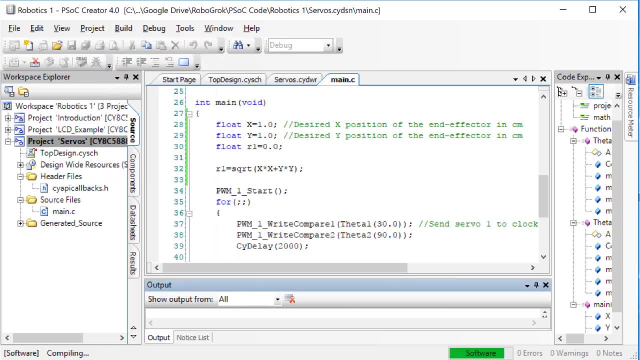 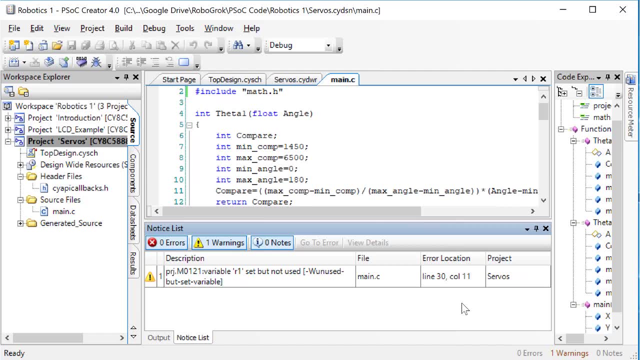 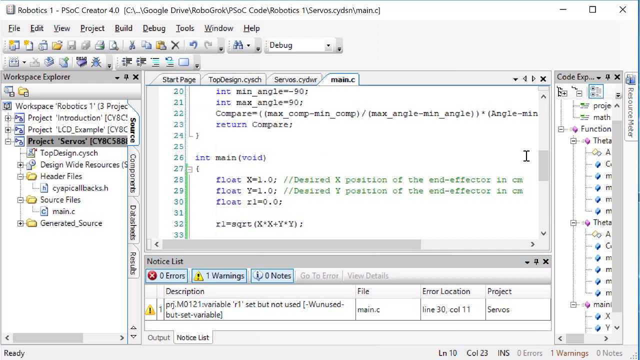 let's go ahead and build this program. now I get a warning that says R1 is set but not used. that's OK because we haven't yet put in the lines that use R1. so as long as you didn't get any errors and you have a 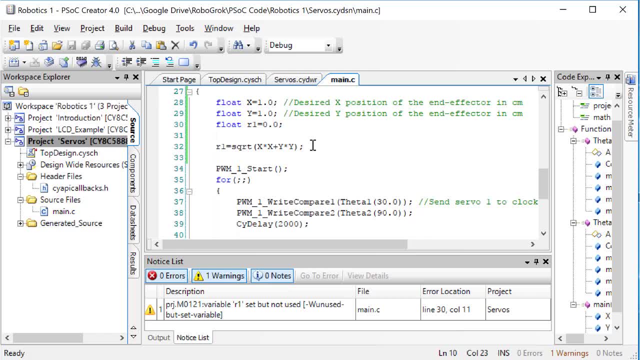 green bar now next to R1, we're still good to go. I'm going to mark this and say that this is equation 1 from our derivation. let's move on to equation 2. equation 2: equation two. equation three: equation: personally, I don't want an equation that saysю: 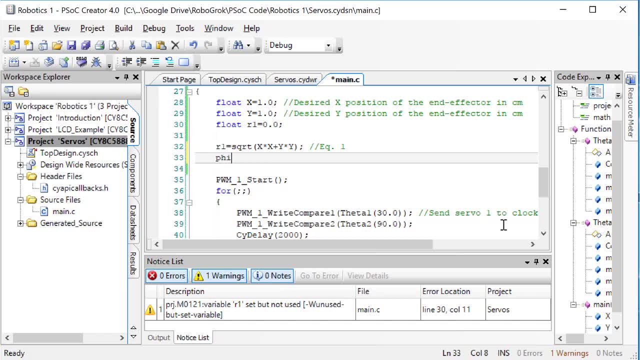 Equation two calculates the value of phi one. We have to use the arc cosine and thankfully that's a function built in to the math library. It is a cos. We're taking the arc cosine of a four squared minus a two squared and I'm going to put some 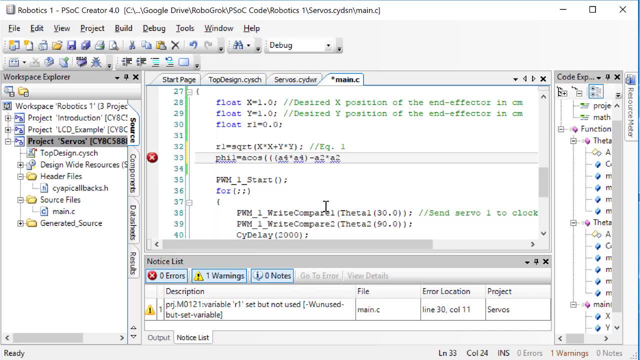 extra parentheses around here to make sure that we are doing these things in the right order. Minus r one, squared, Okay, Okay, Then we have to divide this whole thing by negative. two times a, two times r one. Now we have to make sure that all these new variables that we've used we go back up to. 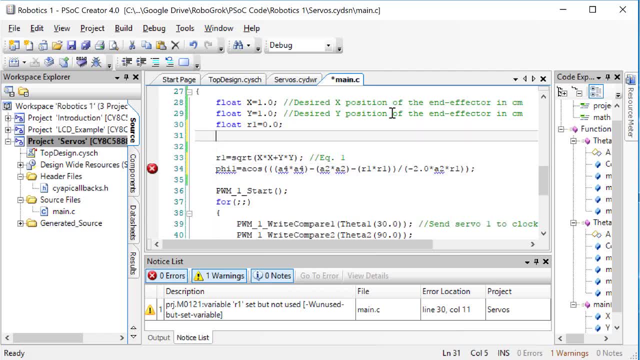 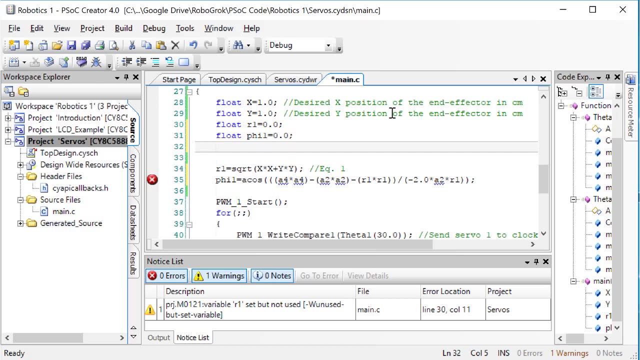 the top and declare them So. phi one is a new variable, Let's do float phi one. Then we need a two and a four. We previously measured a two and a four and put it into our python code when we were doing forward kinematics. 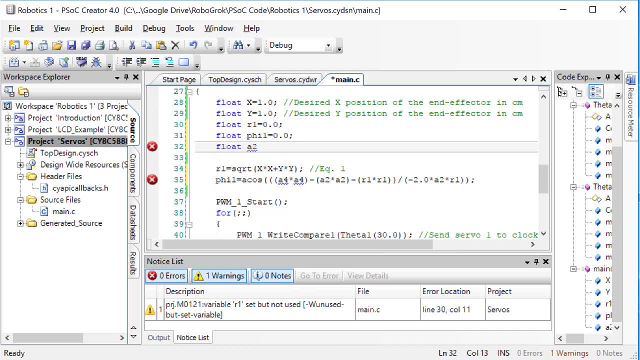 So we don't have to remeasure this again. Let's just use values we got and put into our python code. Okay, Okay, Okay, We've done this already. It's prepared at r, just below r. Okay, how many letters does our python code solve? 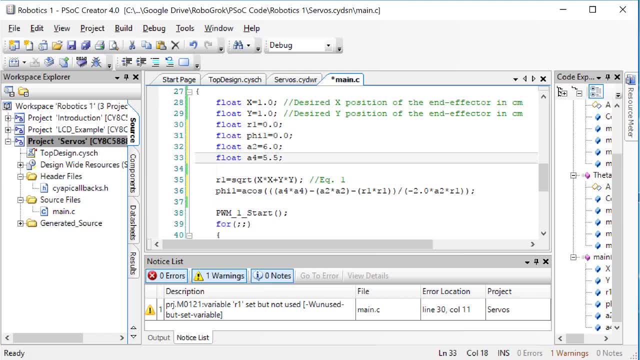 It says 3. 2., 2., 1. 1.. Let's change it. That was a three. It has a question. it can give us an answer. that's that. sorry, I have no clue. Oops, I would do it again differently from here. 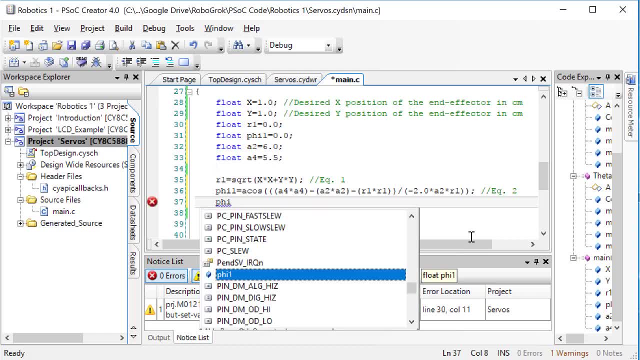 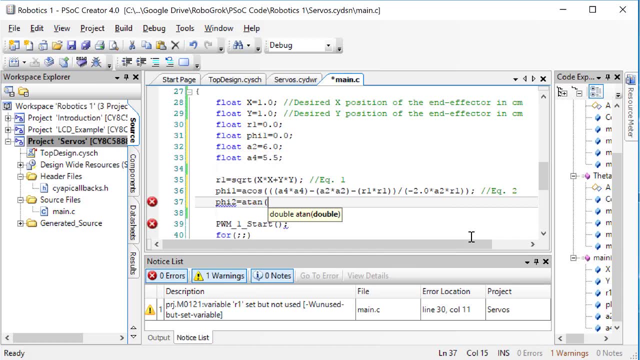 Okay, looks like we're done with equation two. Let's move on to equation three. Let's move on to equation three. Equation 3 calculates phi 2 using the arctangent, So we need to go back up and declare phi 2.. 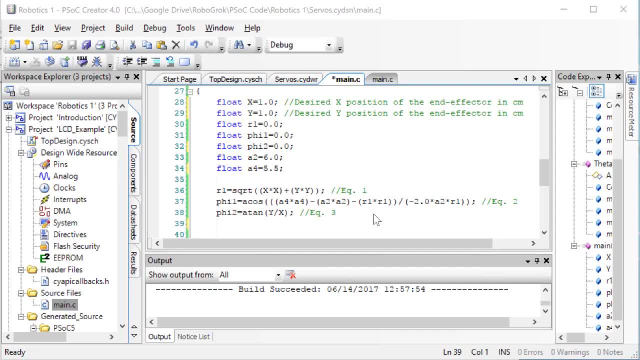 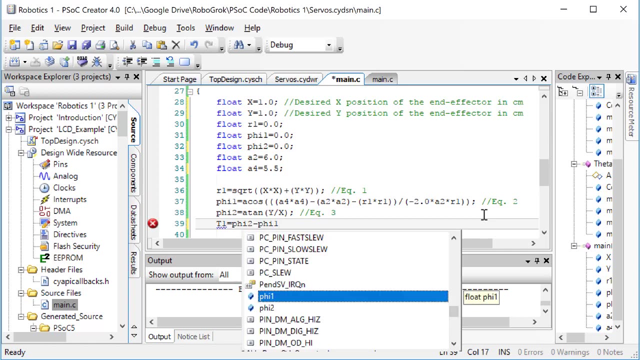 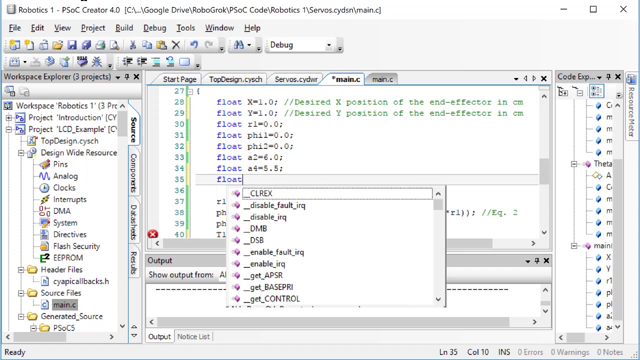 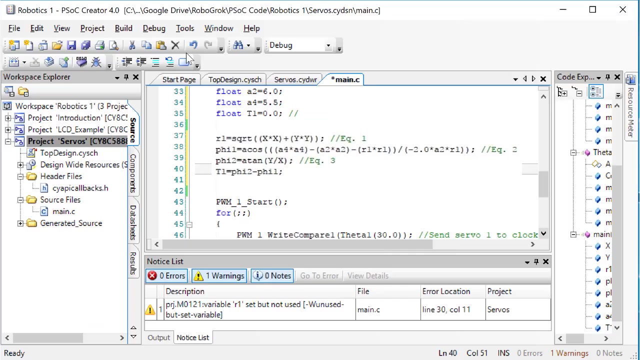 Alright on to equation 4.. Equation 4 calculates T1 by taking phi 2 minus phi 1.. And we have to go back up here and declare T1.. Note that T1 is in units of radians. It's important for us to note that T1 is in radians because our theta 1 and theta 2 functions. 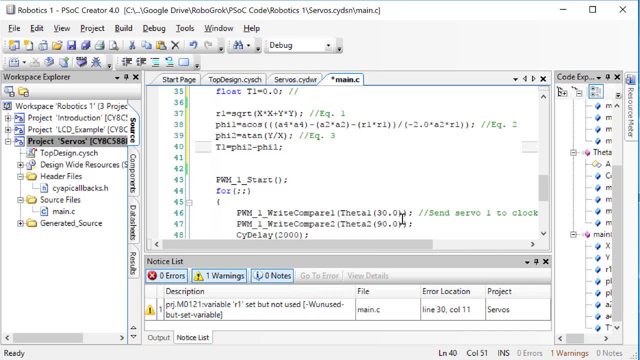 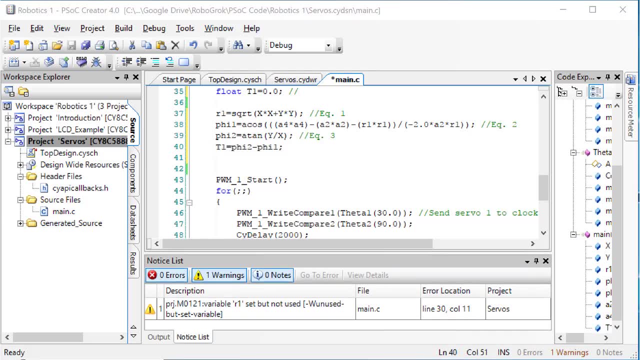 here. Take as input the value of the angle in units of degrees, So we'll need to convert. Okay, on to equation 5.. Equation 5 calculates phi 3 using the arccosine. I'm going to start by copying our calculation of phi 1, since that one also used the law. 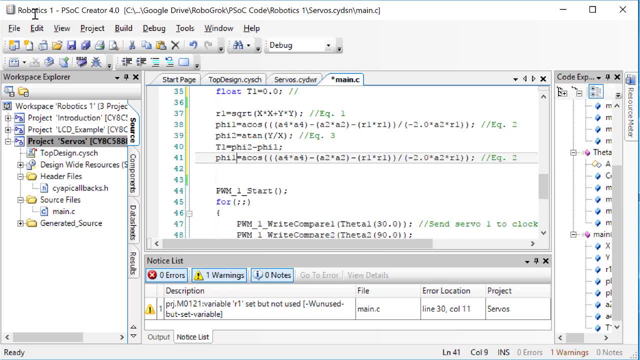 of cosines. This will reduce the number of things I need to type out. Let's change this to phi 3. Then this should be r1 times r1 minus a2 times a2, minus a4 times a4, and then divided by negative. 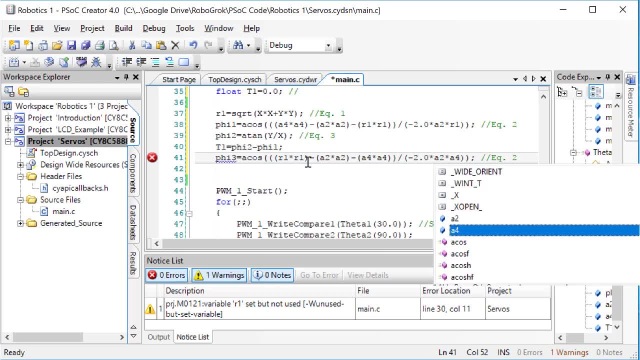 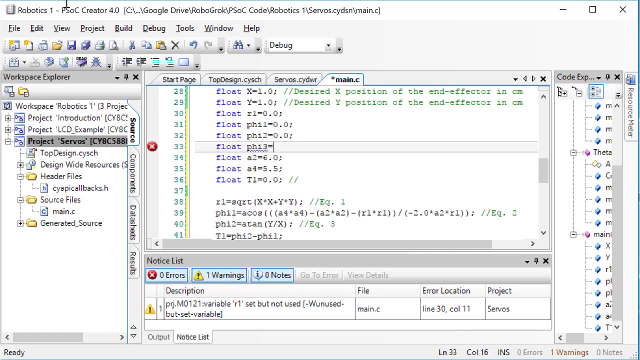 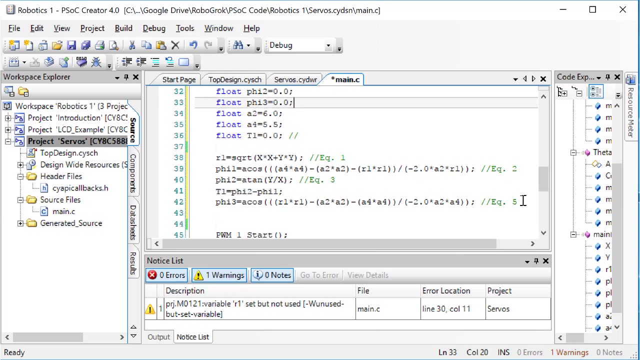 2 times a2 times a4.. There we go. This is equation number 5.. And we haven't yet Declared phi 3.. So let's go up and do that, Float phi 3 like that, And we only have one equation left here. 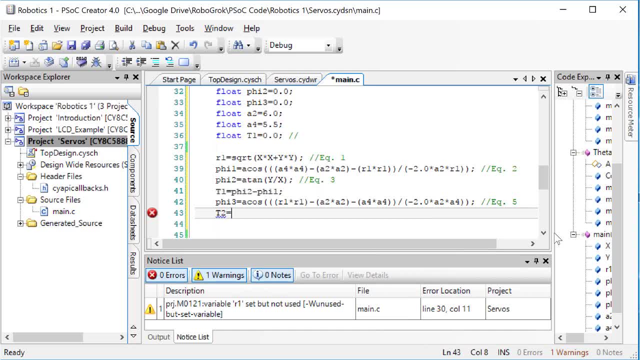 We've got T2 is equal to we put 180 minus phi 3.. However, Let's keep in mind that this phi 3 is actually in units of radians, So I don't want to use 180 here. I better use pi. 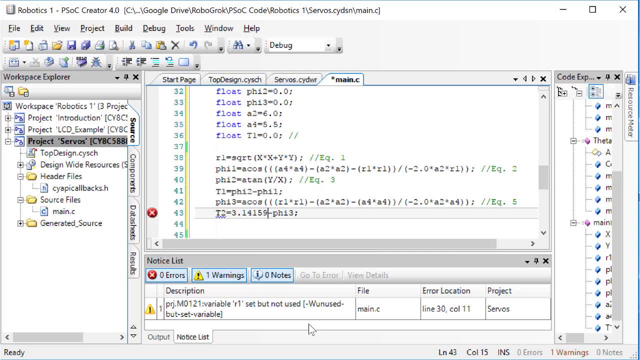 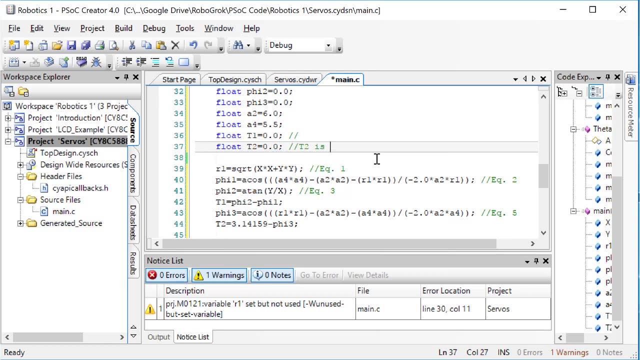 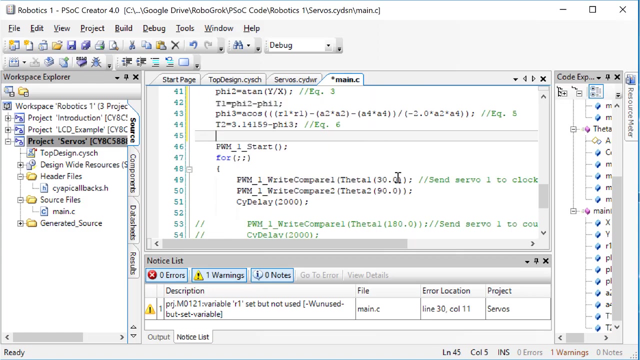 3.14159 will be plenty close for our purposes. Then let's go back up And declare T2.. Okay, Okay, Okay. and now the two angles that we want to send the servos to will be T1,, and we need. 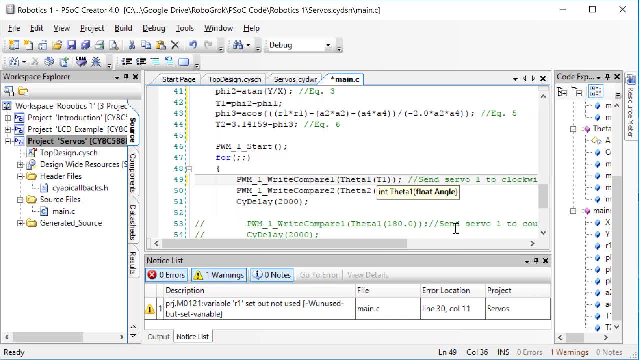 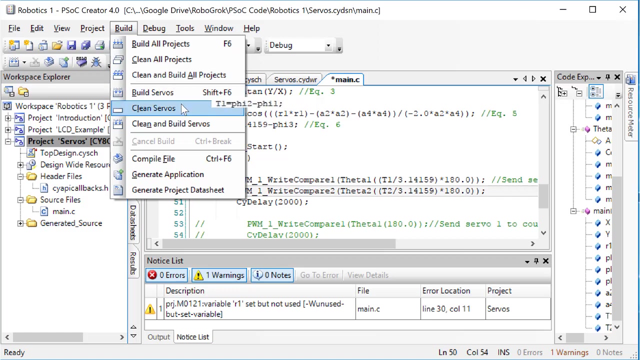 to convert that to degrees. So it's going to be T1 divided by pi times 180.. And we'll do the same here. Theta 2 should be T2 divided by pi times 180.. Let's build this and see if we have it. 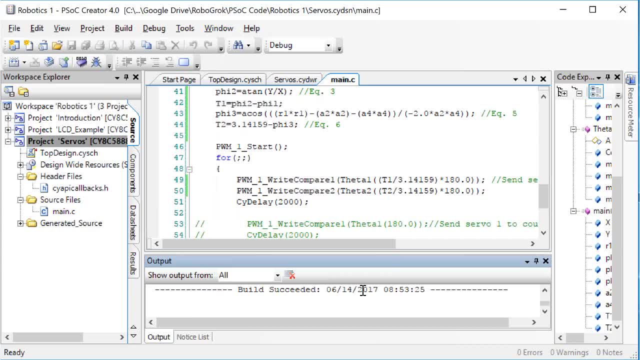 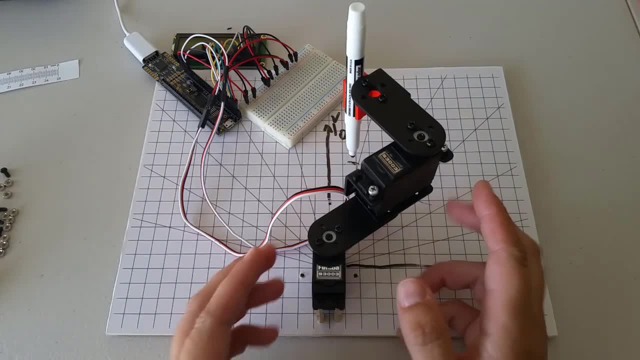 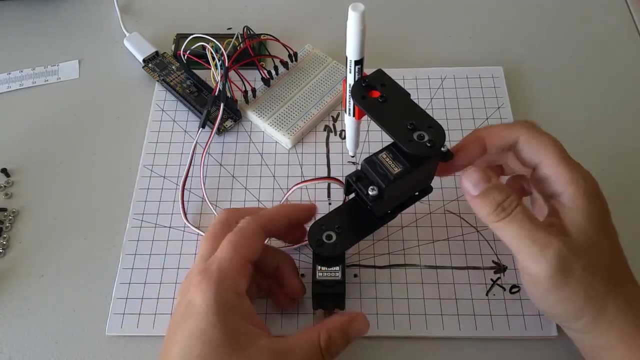 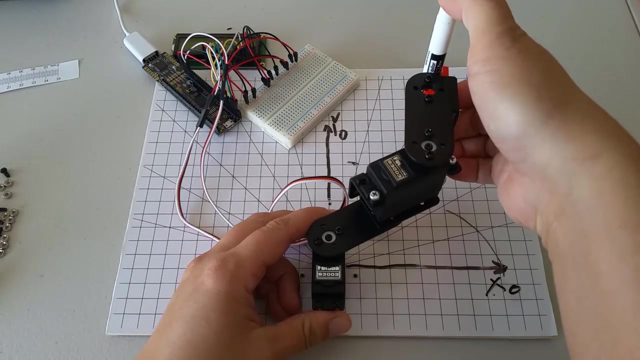 See if we have any errors. Build succeeded. Now back here in our build, we need to make sure that the XY position we're commanding the end effector to go to is a position that actually is within its workspace. So let's start by positioning the end effector in a position that's easy to reach. 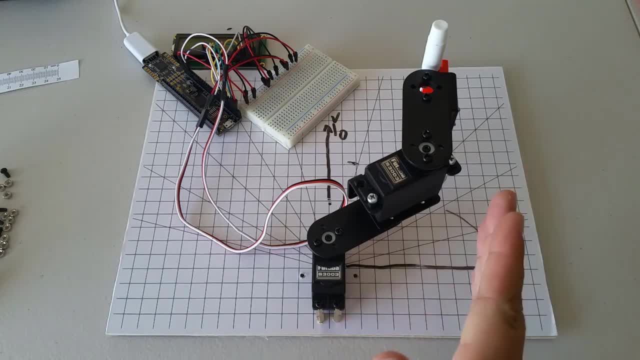 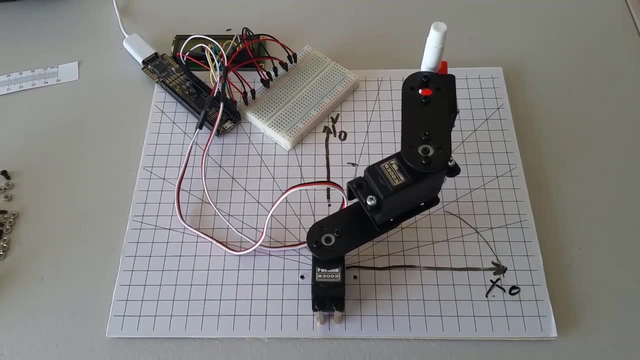 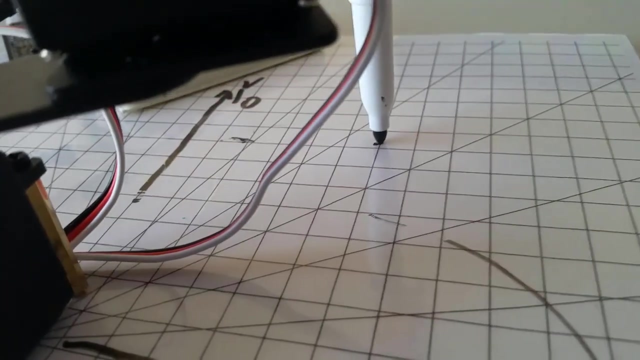 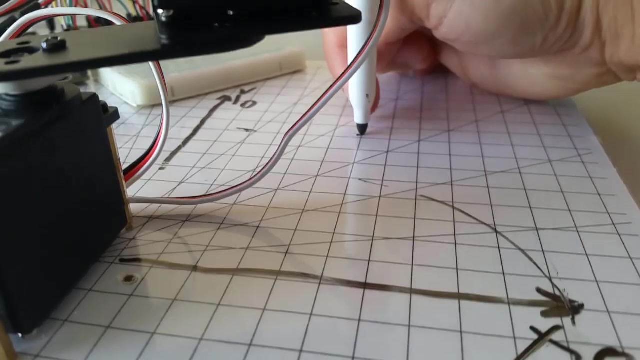 In other words, it's not anywhere near the end effector, It's the limits of the servos. So here's an example of one position that it can easily reach. The X position is 1,, 2,, 3,, 4,, 5, 6.. 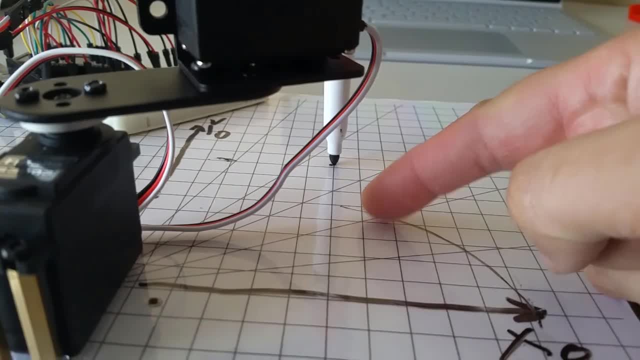 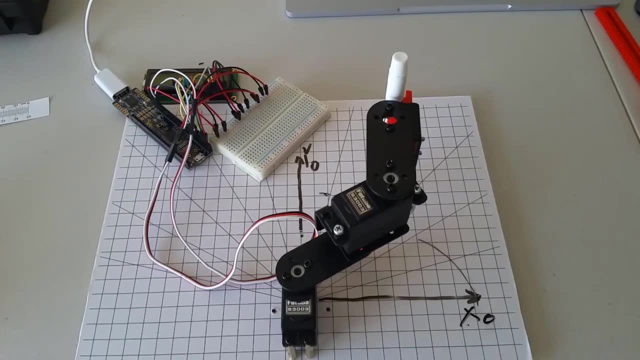 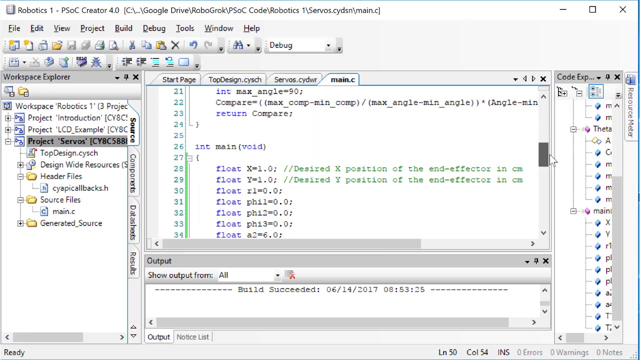 And the Y position is 1, 2,, 3, 4,, 5,, 6,, 7, 8.. We're going to do that. We're going to try to go to 6, 8.. Back in the code, let's enter 6, 8 for XY. 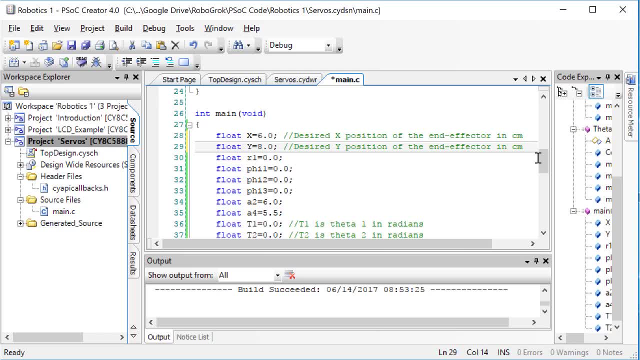 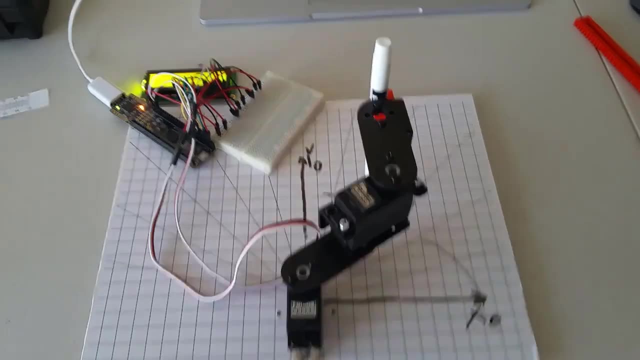 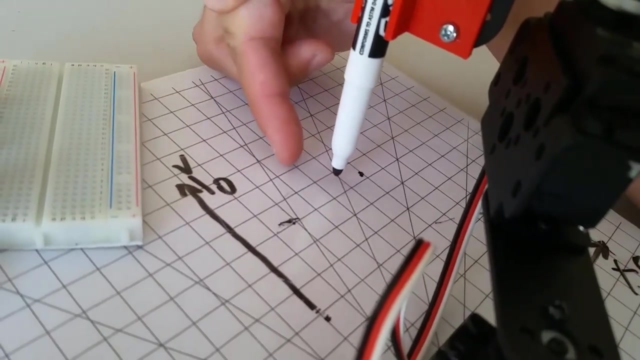 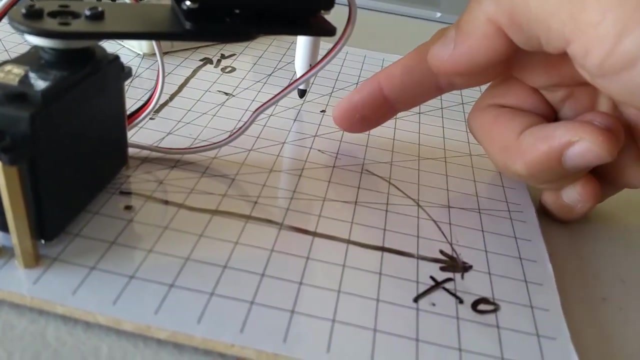 Then log in the USB cable And program the PSOC And let's look at what position the end effector goes to. It went to 1,, 2,, 3,, 4, 5, approximately in X, and 1,, 2,, 3,, 4, 5,, 6,, 7,, 8 point something. in Y. So our X position is: 1,, 2,, 3,, 4,, 5,, 6,, 7,, 8, point something in Y. So our X position is: 1,, 2,, 3,, 4,, 5,, 6,, 7,, 8, point something in Y. 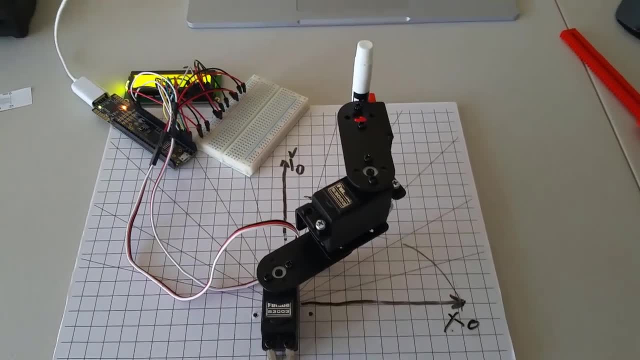 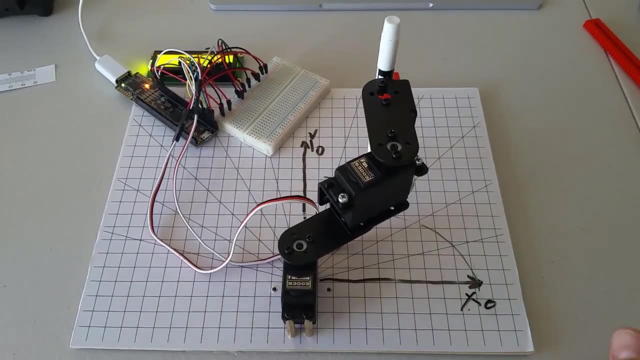 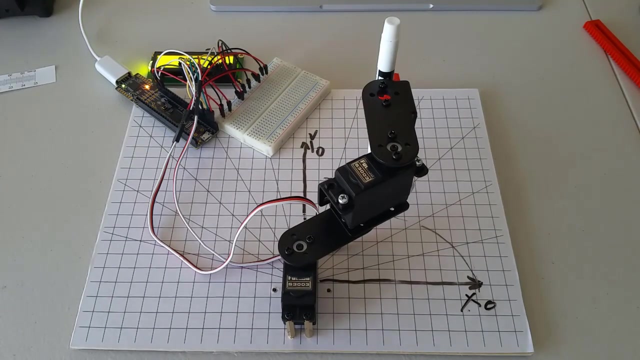 So our X position is off by about a centimeter And our Y position is off by a fraction of a centimeter. Let's try another position. Let's see if we can get the end effector to move 2 centimeters to the right of where it. 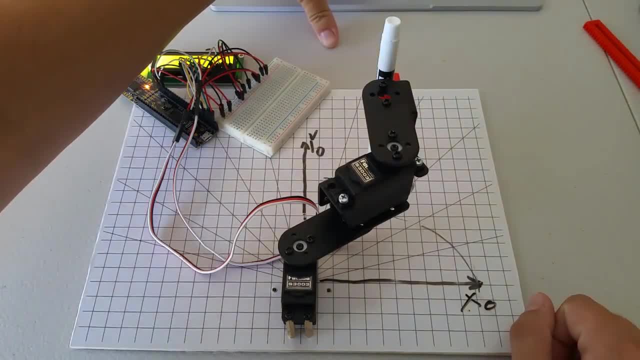 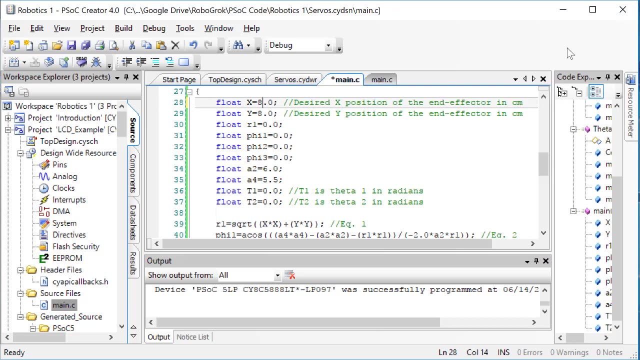 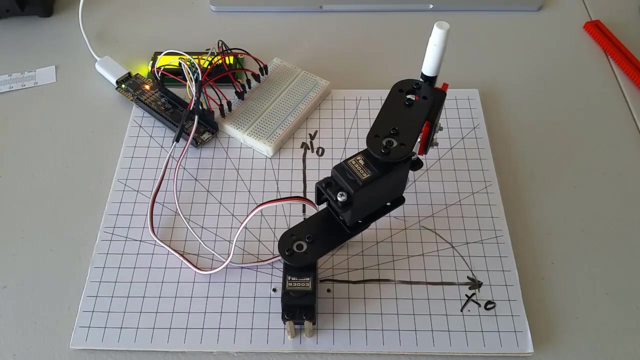 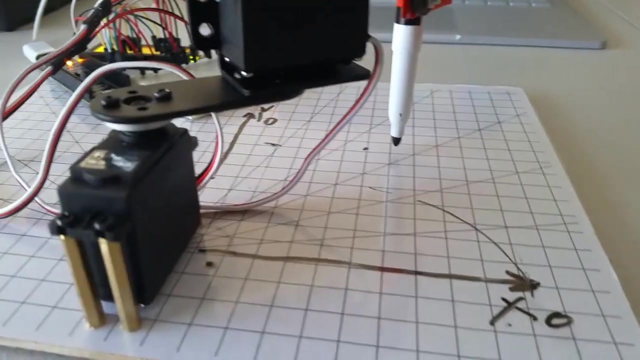 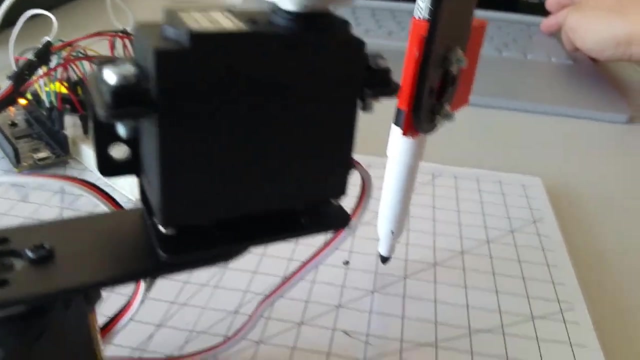 is right now. Change X equals 6 in your PSOC code to X equals 8.. And then program the PSOC. It did move about 2 centimeters to the right. Let's try and move it back to the left. We'll change the X from 8 back to 6.. 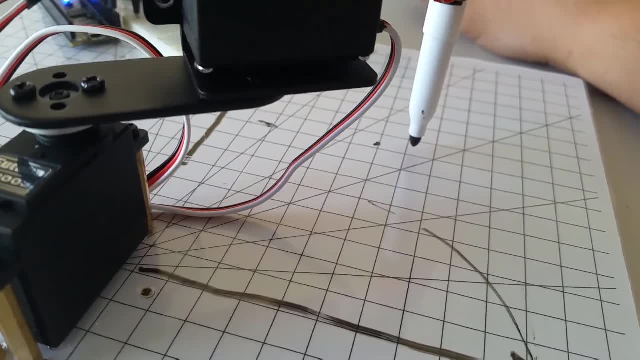 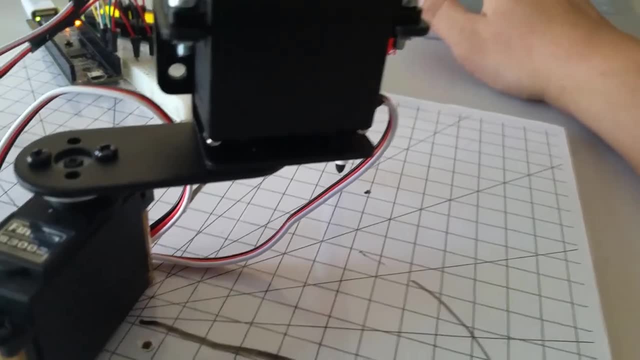 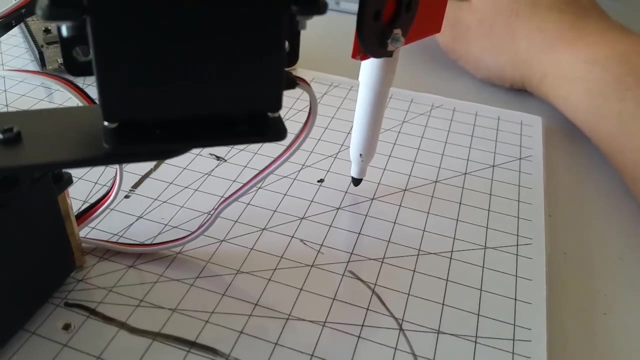 Program the PSOC And then program the PSOC, And then program the PSOC. There we go. And now let's go back again. Change the X to 8. Let's see if we can make it go 2 less in Y. 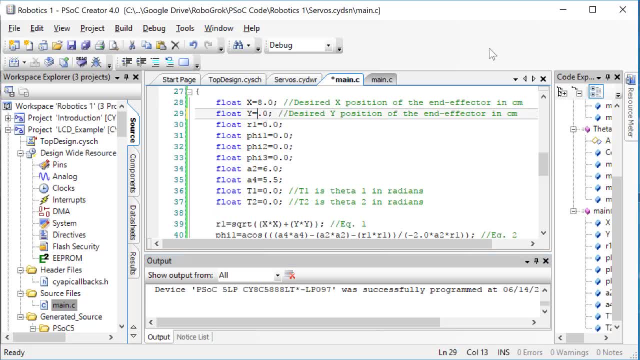 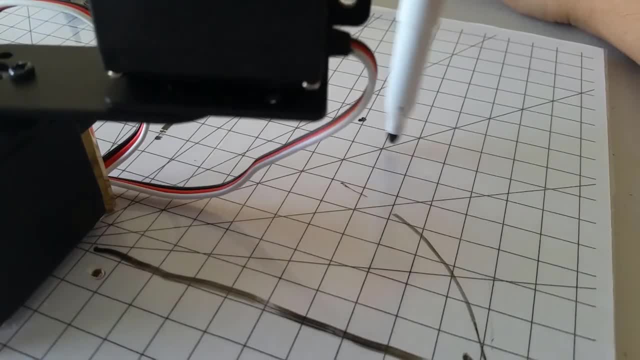 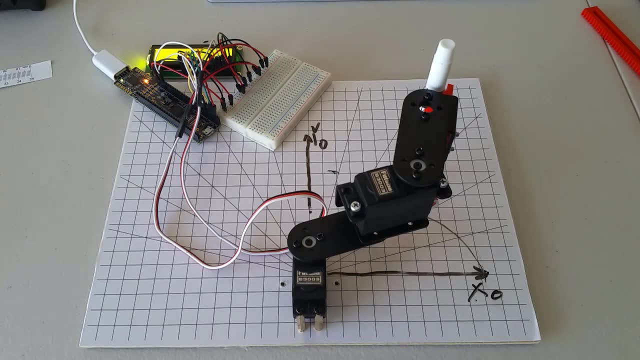 Let's change Y to 6.. Okay, We got it. We're back to where we started. We're starting to get the depth. Let's try and make that happen again. Let's see if we can get this to go back to the right. 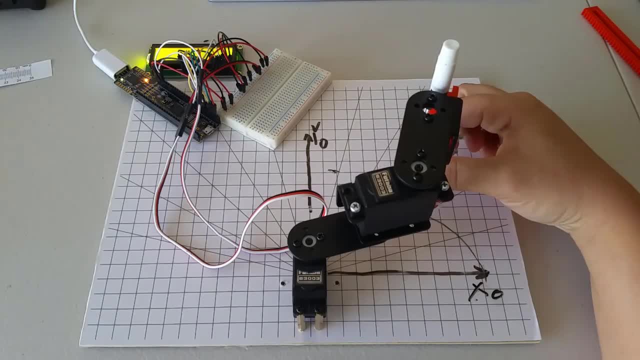 Let's try. We're back to where we started. We're talking about the X mark And we're going to have some depth. Now, keep in mind that you can't try to go to an XY position that is, outside the robot workspace.